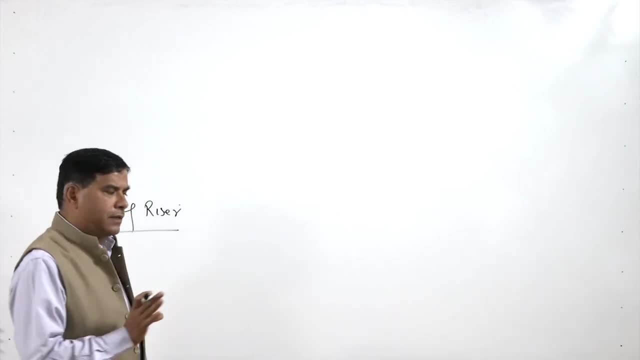 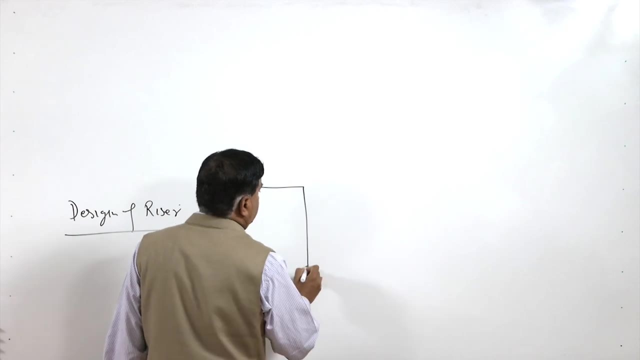 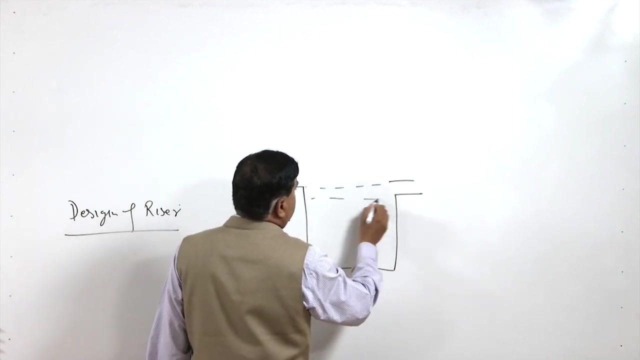 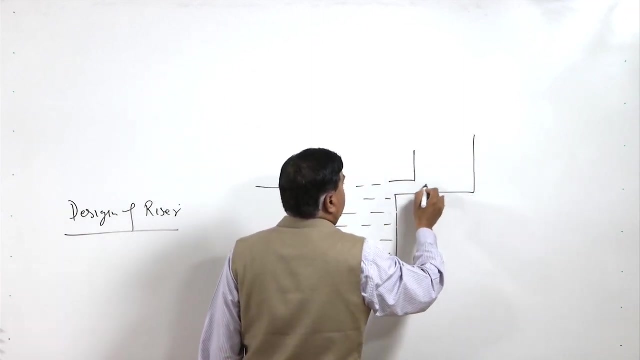 mould so that the shrinkage related with the liquid to solid state transformation can be compensated. But to perform this role, say, this is the mould and here we have riser. So if any shrinkage is taking place due to this transformation from the liquid to the solid state, that need to be compensated by feeding the molten metal. 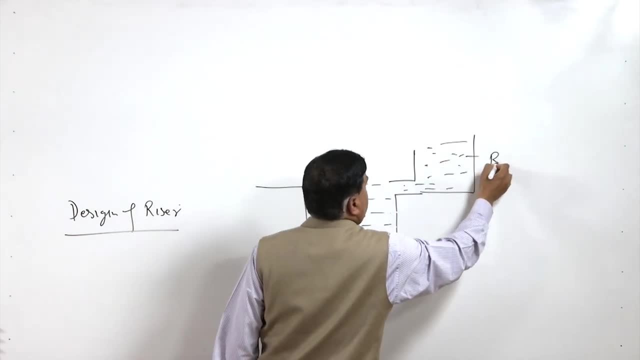 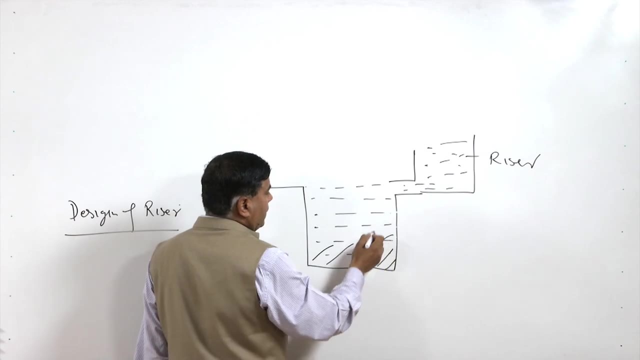 present in the riser. So this is say riser. So it is expected that the solidification of the molten metal will be taking place first in the mould. So, and once this solidification is over, then whatever shrinkage due to this transformation. 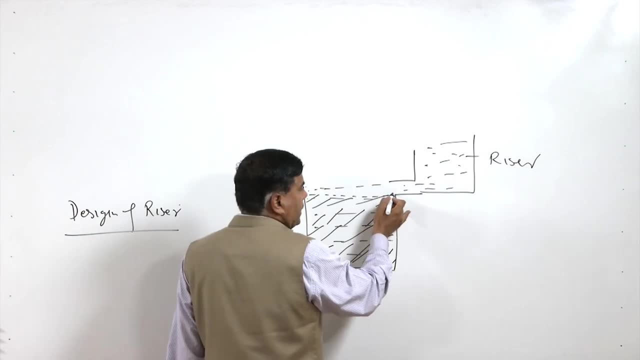 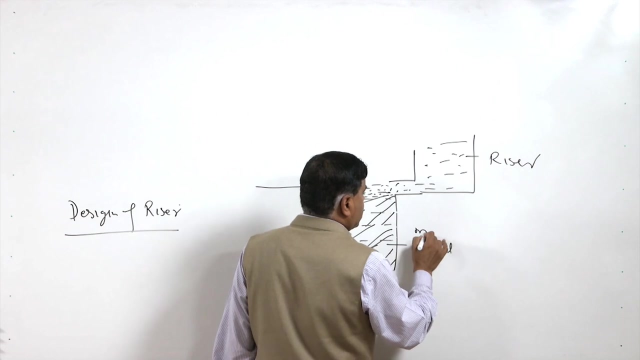 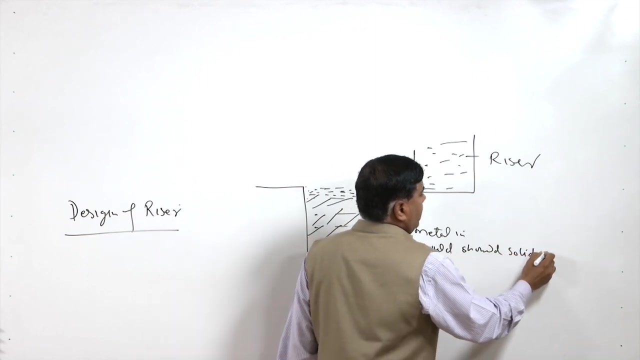 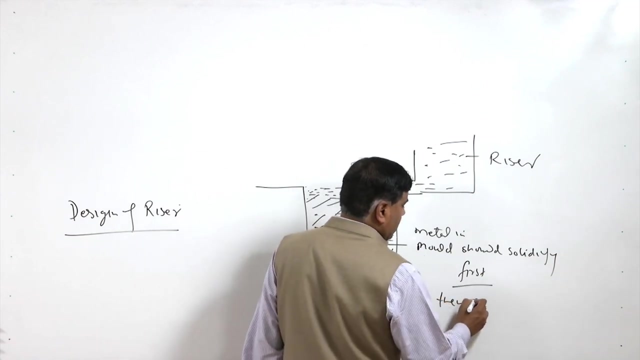 has occurred, that will be left at the top. So that shrinkage, that volume of the metal which is deficient due to the shrinkage, is to be fed from the riser. So the mould, or you can see the metal in mould, should solidify first and then solidification in riser should. 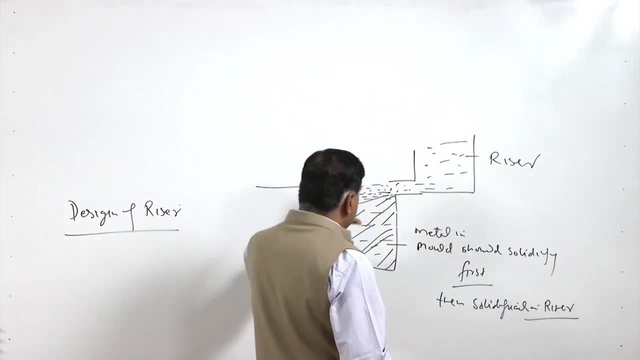 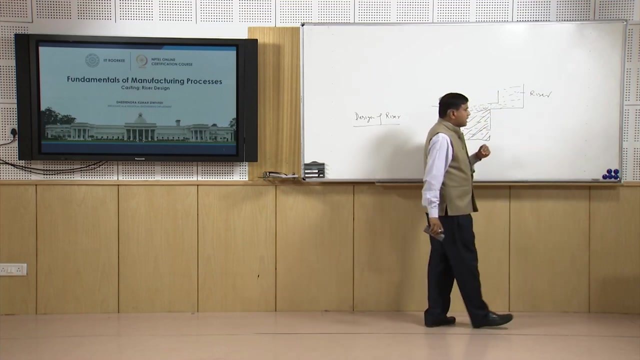 occur means till thus molten metal. until the molten metal solidifies means the structure is solidifies, So molars. ok. So all right, I will be leaving that there and we will continue the meeting. Yes, So the molten metal should solidify in the mould first and so that, whatever is the shrinkage, 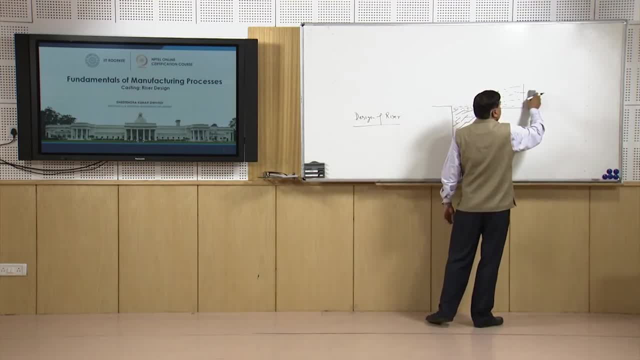 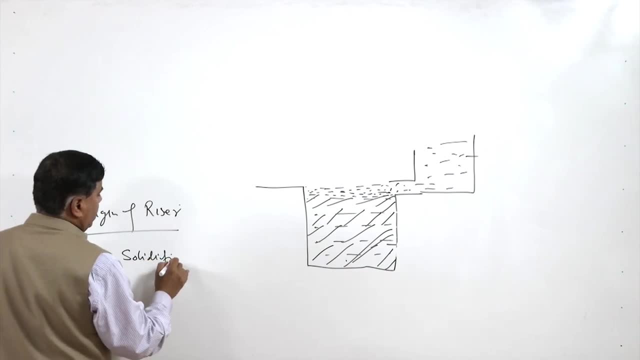 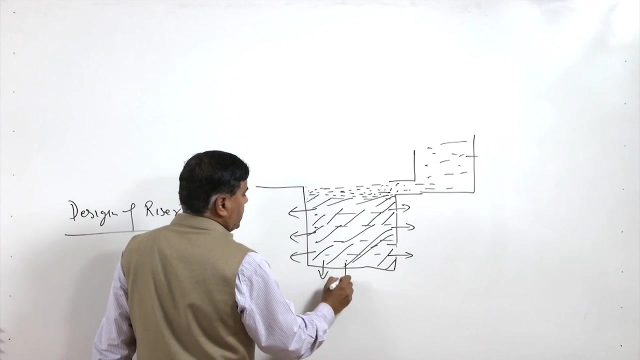 is there that can be fed in by the molten metal in the riser. So this solidification- we know that the solidification of molten metal depends upon- and the fact that how fast heat is transferred from the molten metal to the mould wall. 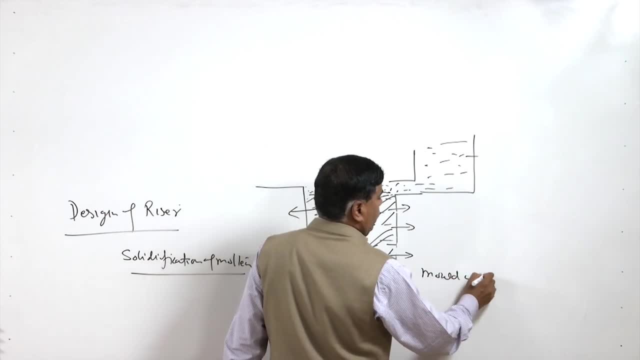 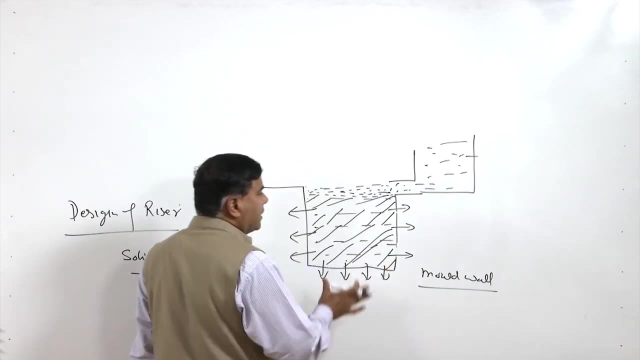 So all around we have mould walls. So if these are of the metal, then they will be extracting heat at much faster rate as compared to the case when they are made of the sand mould. the walls are made of the sand or the moulding sand. 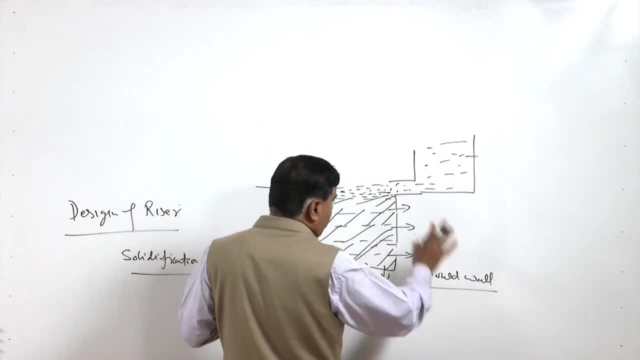 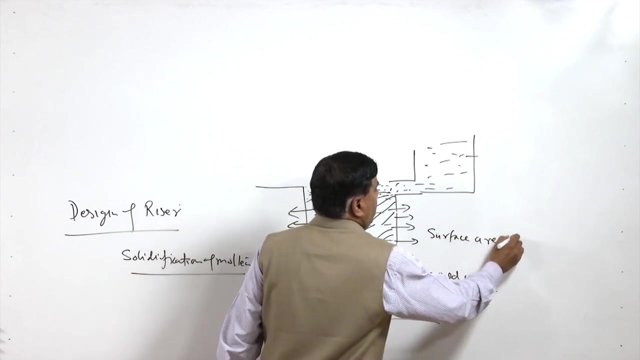 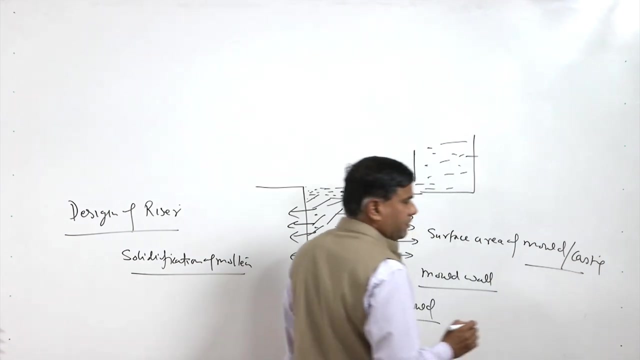 So, in addition to that material aspect, See for a given sand mould. the rate at which heat will be transferred will depend upon the surface area of the mould, or we can say casting, which, after the solidification of the molten metal, will be getting. 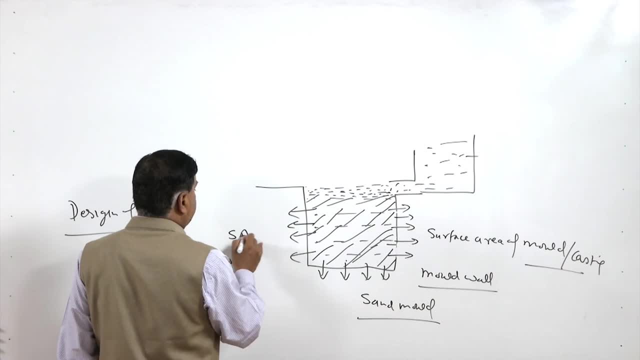 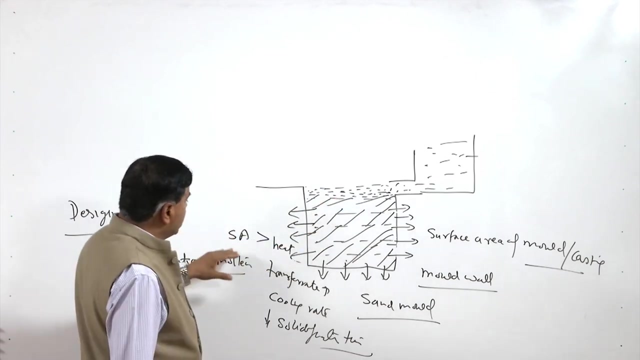 So greater the surface area. surface area is more Then, So the heat transfer rate will also be high, which will be leading to the high cooling rate and so less solidification time. So what we want? that to ensure the solidification of the casting first, it is necessary that 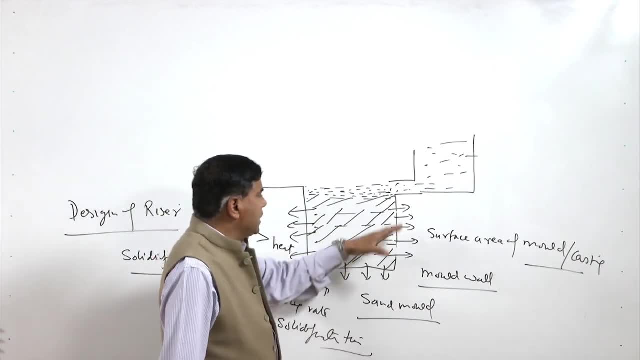 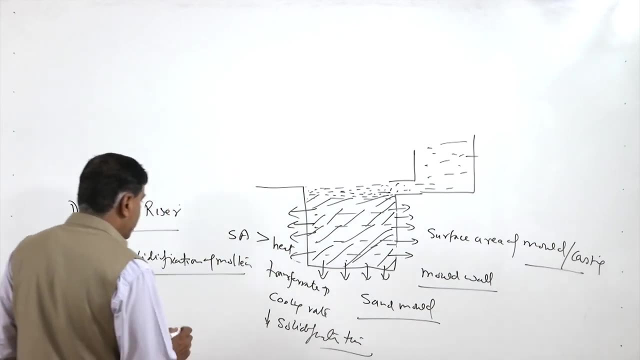 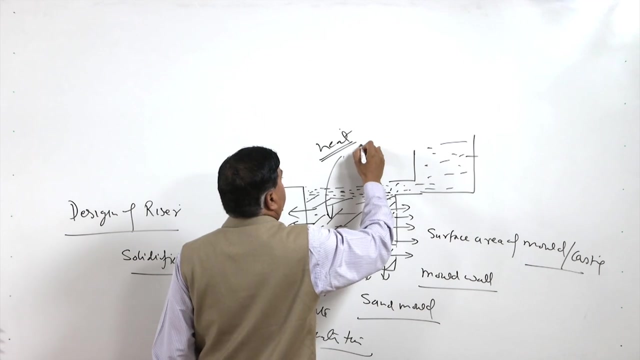 the surface area of the casting is more, So that means the coal rising is more than the surface area of the riser. But in addition to that, we have to consider one more aspect, that is about the volume, since the heat contained by the molten metal depends upon the volume of the molten metal. 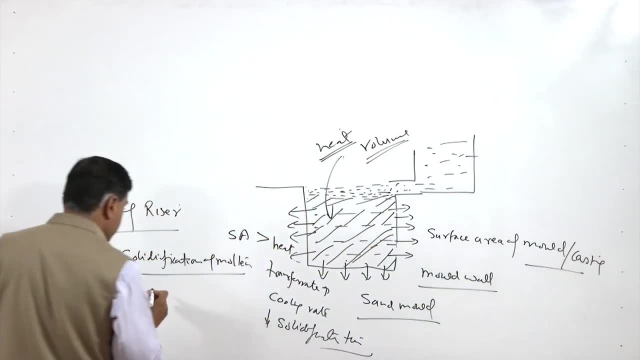 So the ratio of the surface area, surface area to the volume, This is the ratio. This is determining that heat transfer and this is about the heat content. So if the surface area to the volume ratio is high, then the heat transfer rate will be. 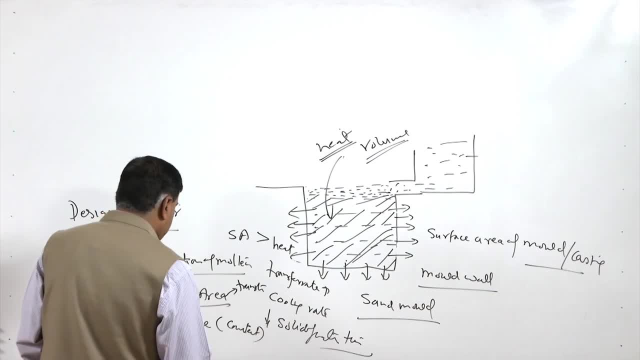 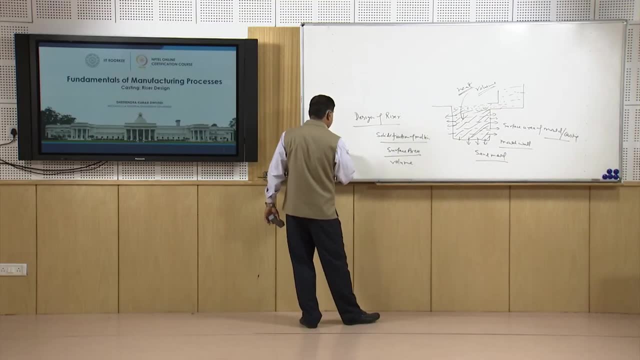 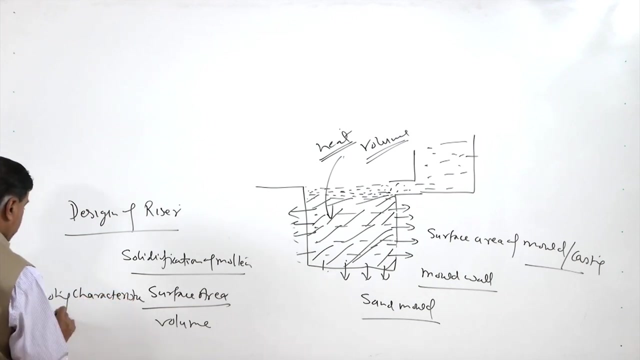 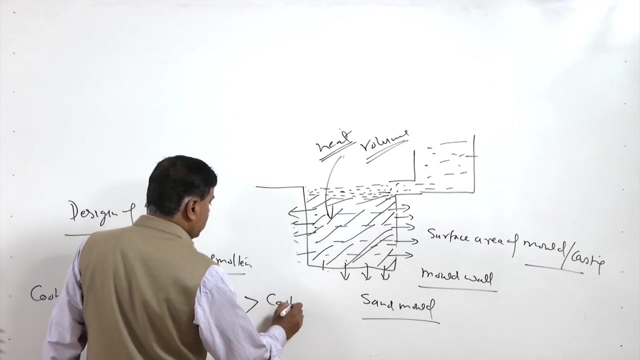 much faster and the cooling will be occurring much earlier. So this ratio is basically used to define the cooling characteristic, cooling characteristic of the mould or of the casting. So if the cooling characteristic of the casting is high, it is higher than the cooling characteristic. 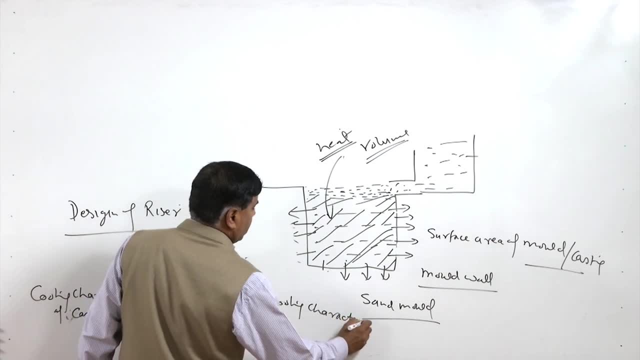 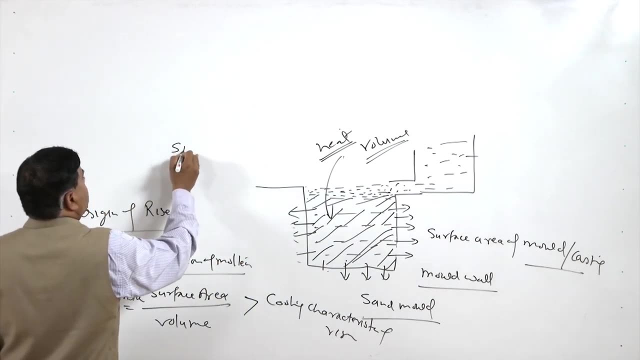 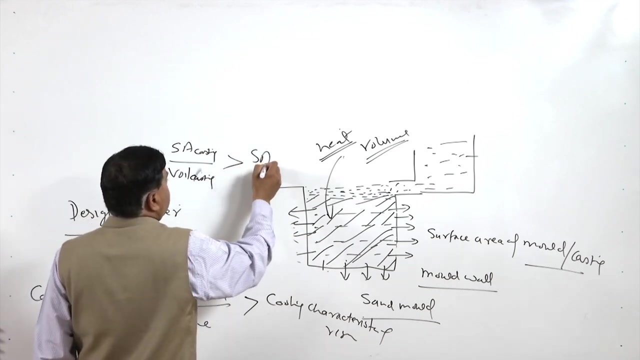 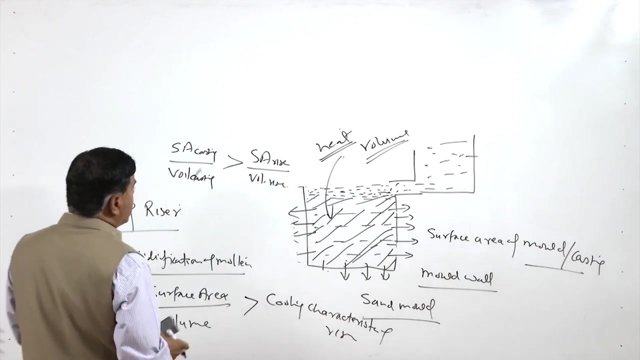 of the mould. So what we can say here? surface area of the casting divided by the volume of the casting. This ratio should be greater than the surface area of the riser. to the surface, to the volume of the riser. If this ratio is high, 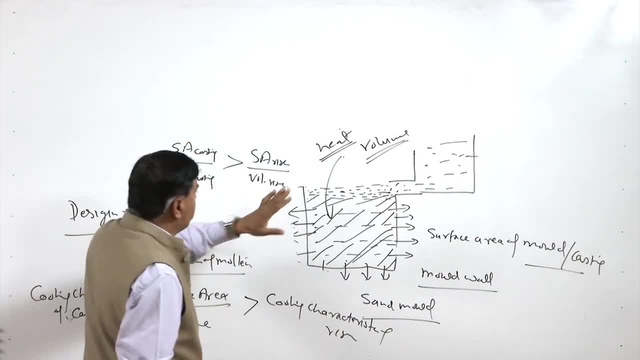 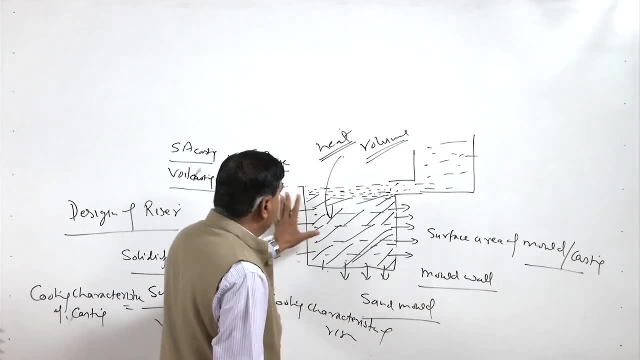 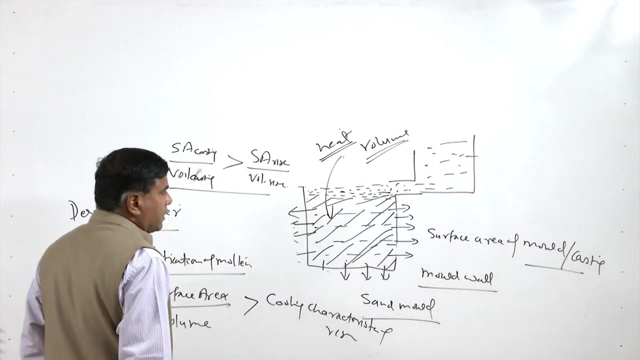 And achieved then means the riser is prepared in such a way that this ratio is obtained, then this will be ensuring that the cool casting will be solidifying earlier as compared to the solidification of the riser. means the molten metal in the rise. molten metal will 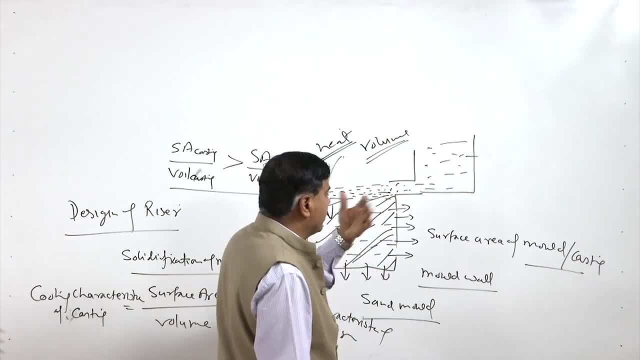 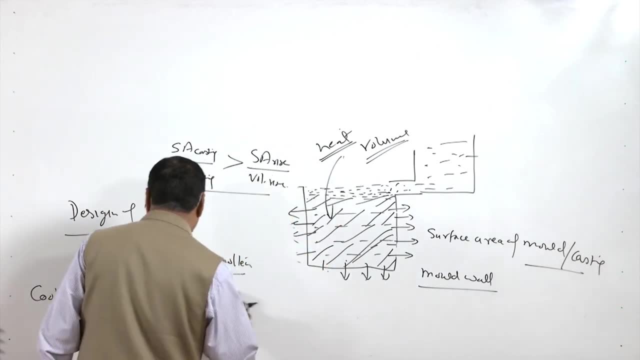 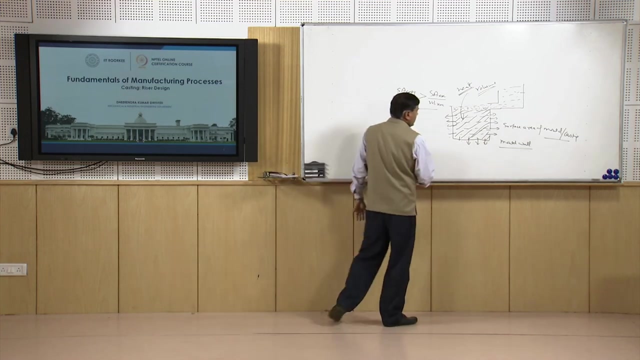 and the metal in the riser will remain in the liquid state for the longer period, as compared to the case in the mould Or For the casting. So the cooling characteristic is one of the important characteristic related with the design of the risers. 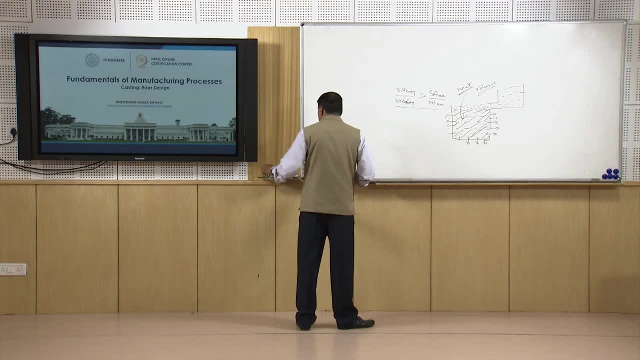 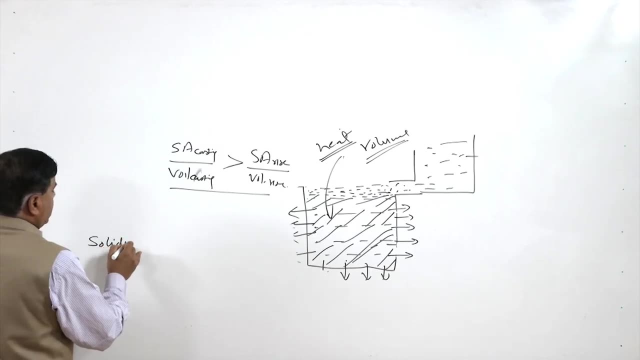 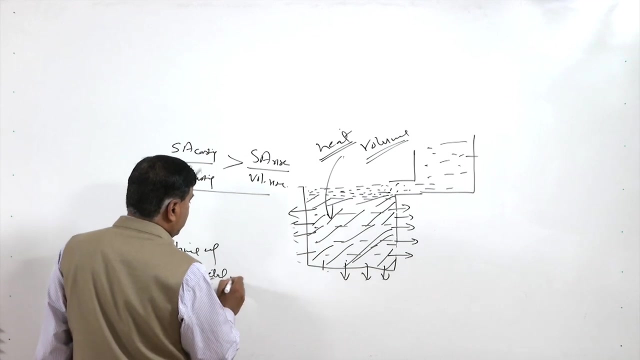 So this efforts have been made to relate the solidification time. solidification time of It can be say in casting or in the riser. this can be given with the help of like, say Tc in Ts in minutes means solidification time in minutes. 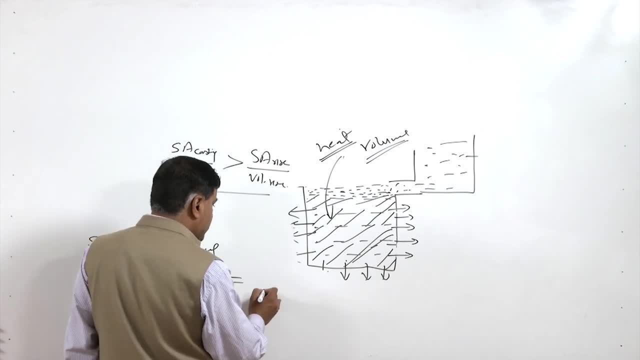 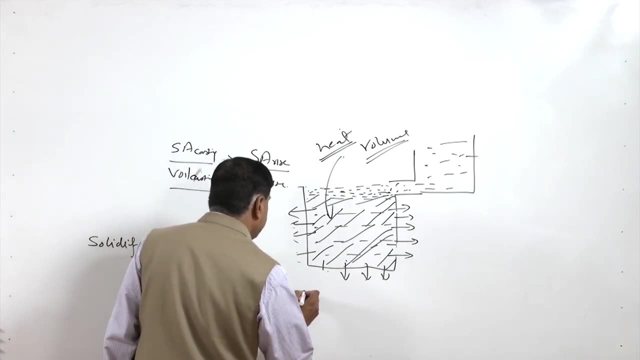 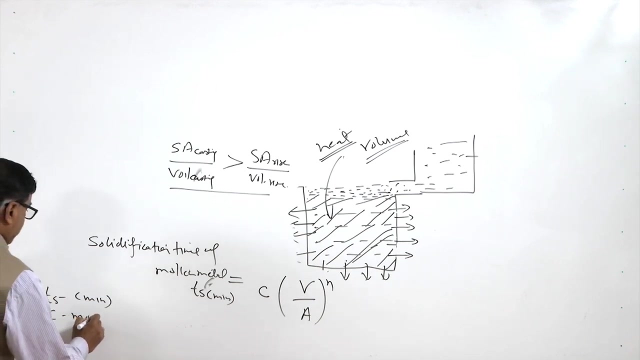 So here, what we have mentioned, like the C is the mould constant and it is the ratio of the V by An. so what are these parameters? are the solidification time? Ts is given in minutes. C is the mould constant. It depends on the thoroughness. 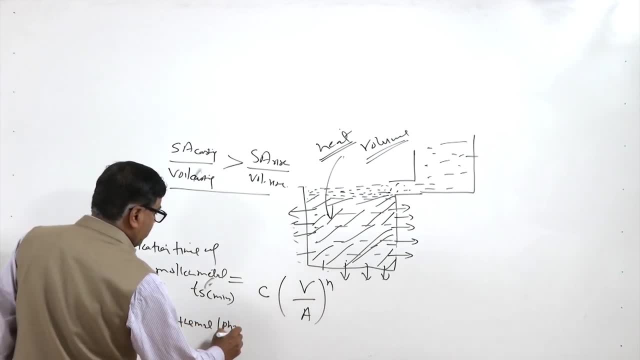 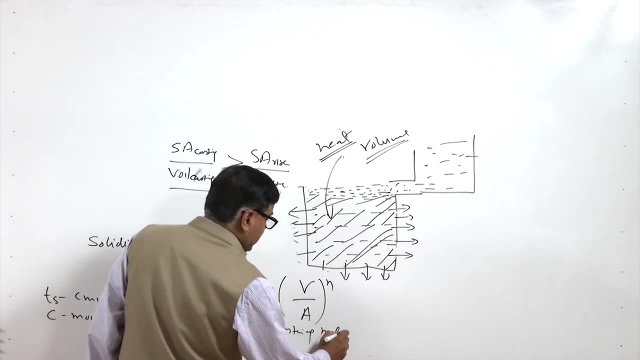 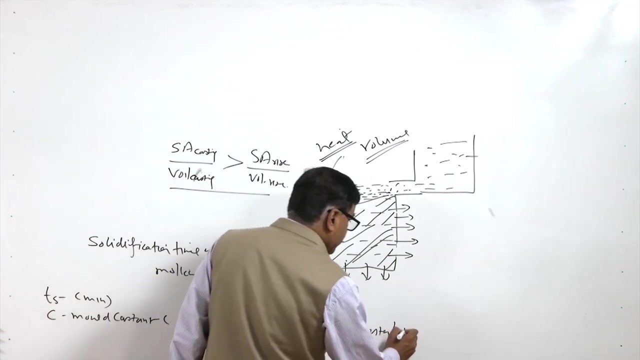 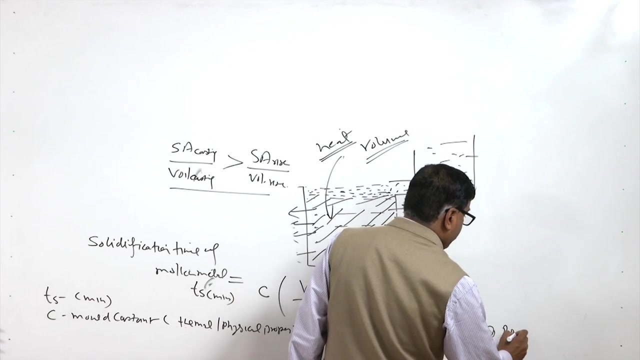 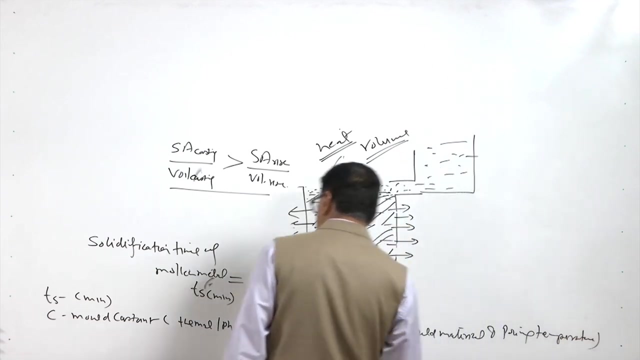 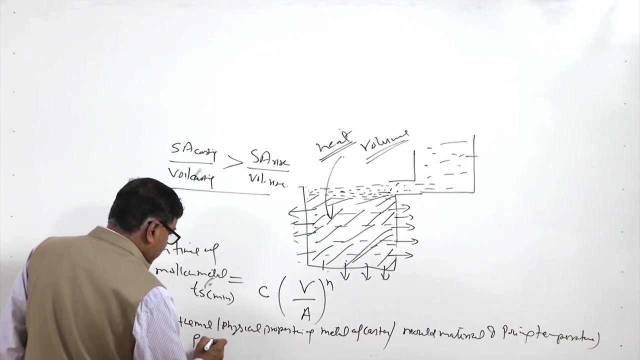 So thermal and physical properties of the metal of casting, as well as thermal and physical properties of the mould material, as well as the pouring temperature, at what temperature molten metal is being poured. So these are the factors which will be affecting- among these, like mainly the row, density, the 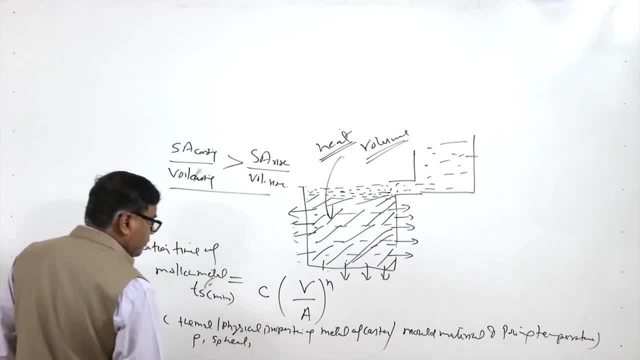 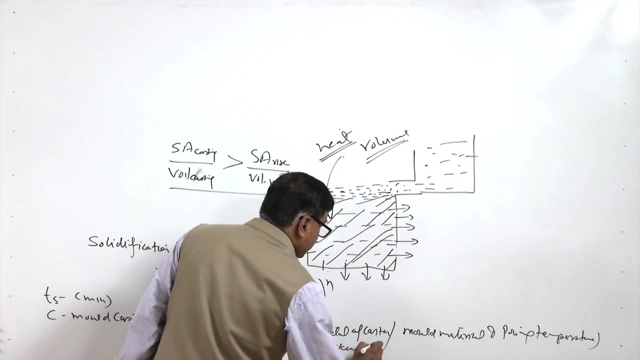 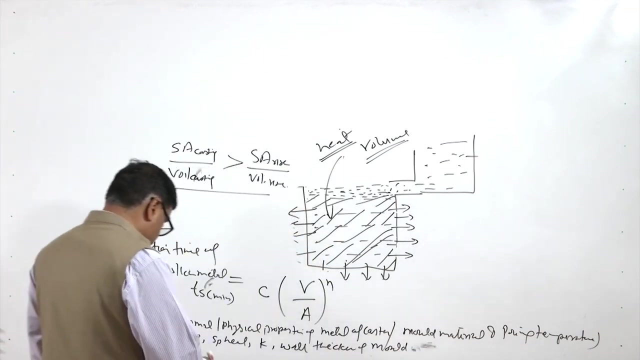 specific heat, thermal conductivity of the molten metal, of the metal of the casting, as well as the mould and wall thickness of the mould wall. Okay, This is what we can say. the V is the volume. V is the volume of the metal, whether it is. 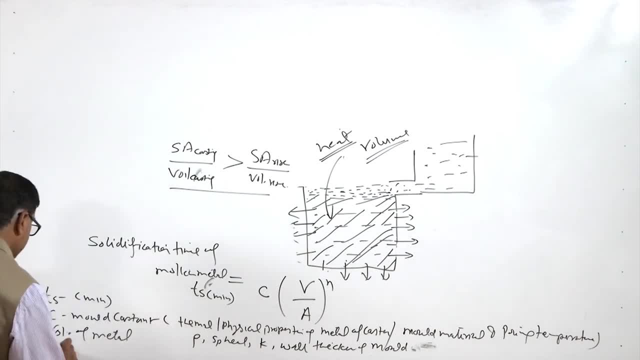 casting or the riser, and A is the surface area of the casting or of the riser. So V is the volume centimeter cube and area in the centimeter square. Square means the mould constant and the Ts is the time for the solidification. 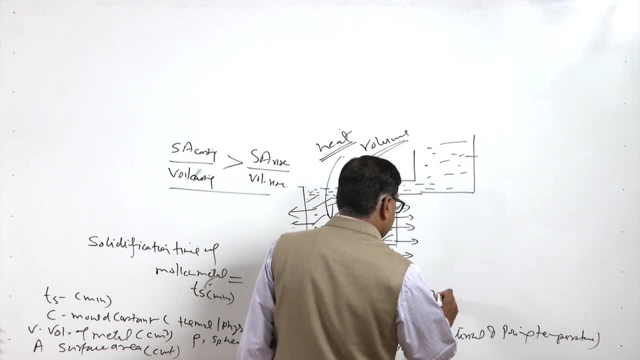 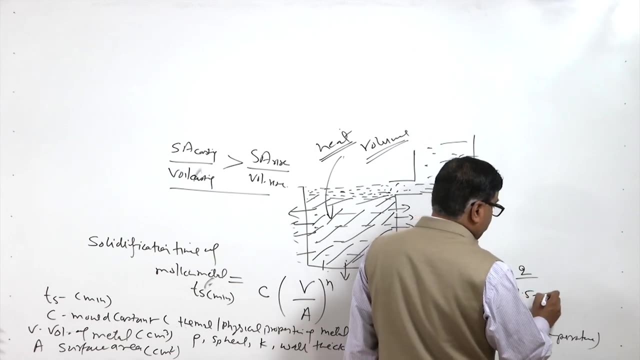 So, and the value of An An is also constant and whose values? normally it is written 2, but it is found in the range of 1.5 to the 2.. So normally it is like solidification time is given as a proportional to the square of. 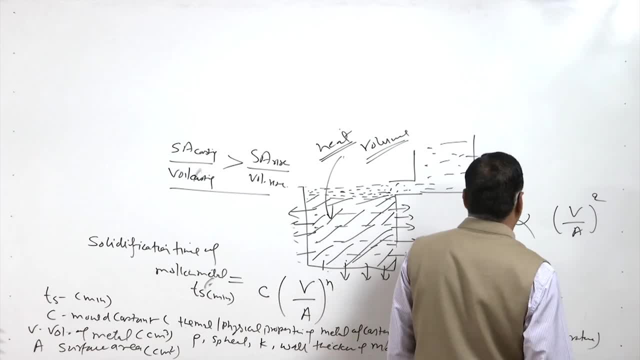 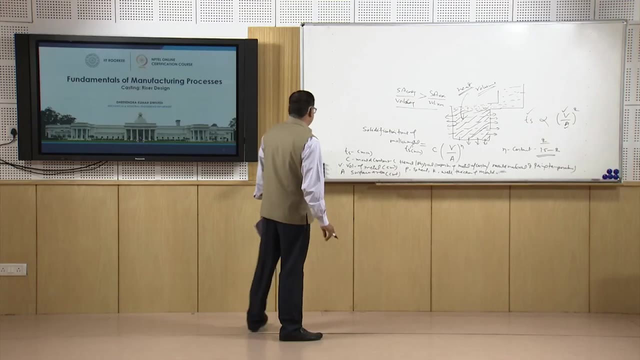 the volume to the surface. So here, for the larger volume, the time will be more. similarly, for the larger area, for a given volume, the time will be less. This is how the solidification time can be given, and this is one of the very commonly. 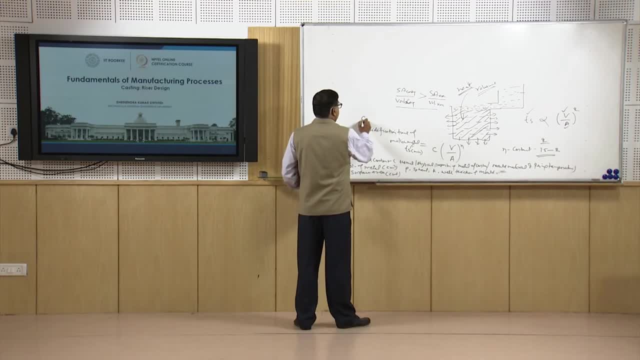 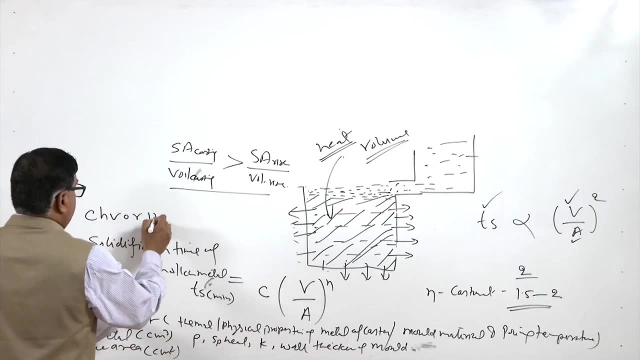 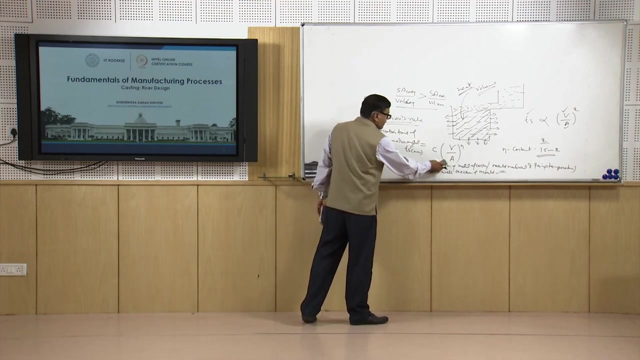 known equation. This is called expressed as CHVOR Okay I N O V S rule used for expressing the solidification time and using this basically, we can determine when the solidification in the riser and when the solidification in the mould will be taking. 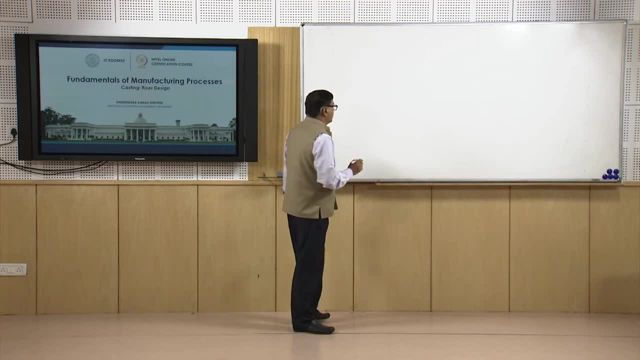 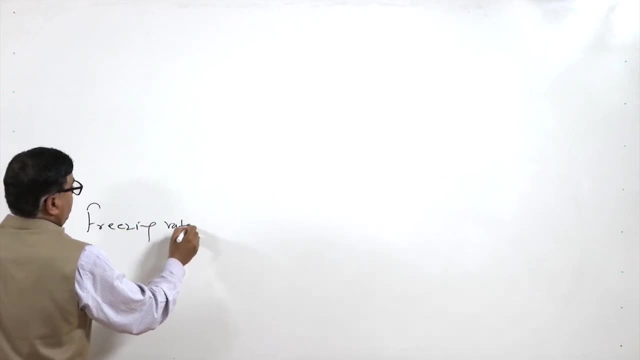 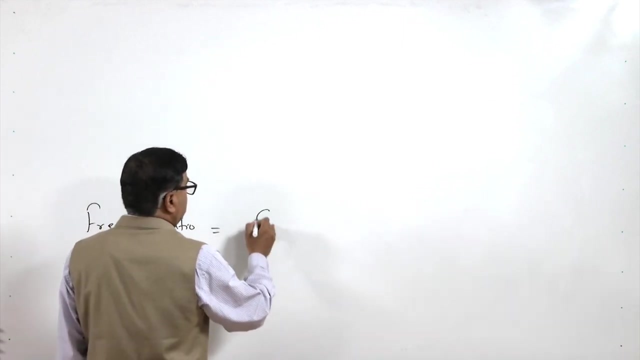 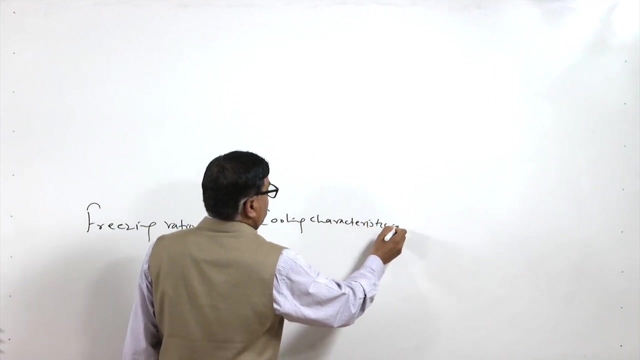 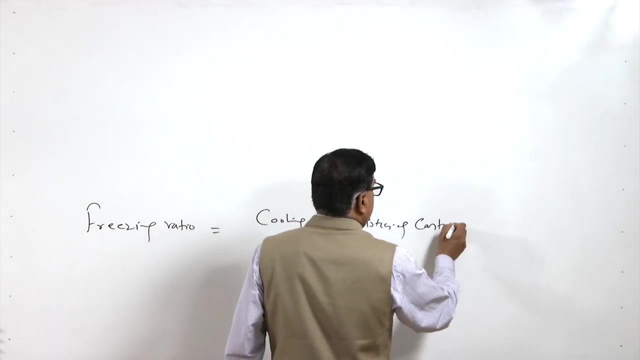 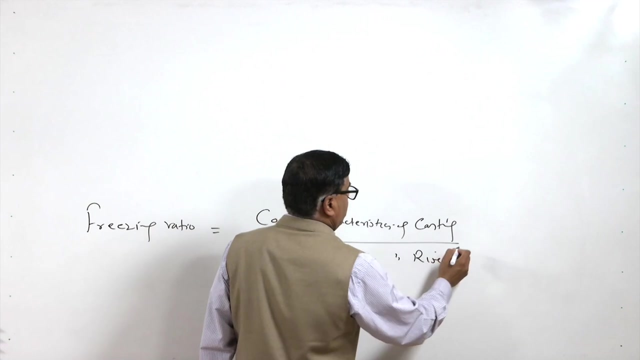 place To express it more clearly, the one term which is called freezing ratio. Okay, So this is the one term which is called freezing ratio. Okay, So this one term also has been obtained or developed, which is basically the ratio of the cooling characteristics of the casting to the cooling characteristics of the riser. 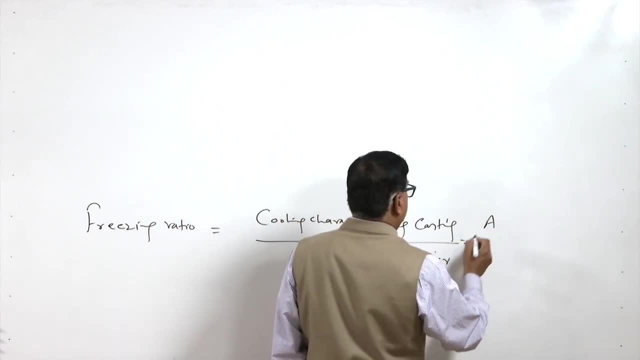 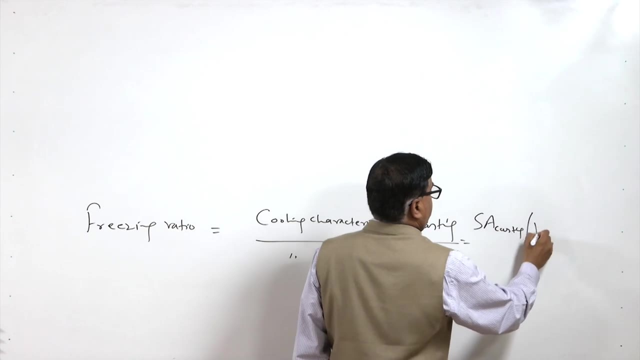 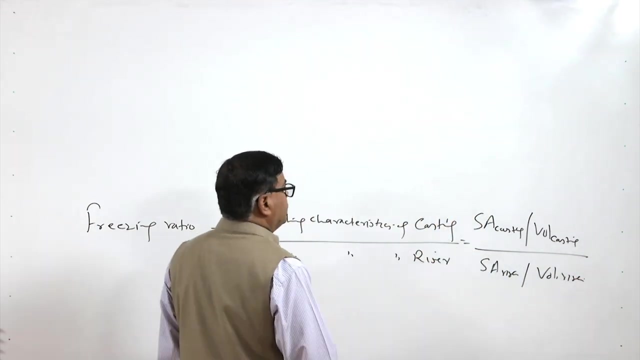 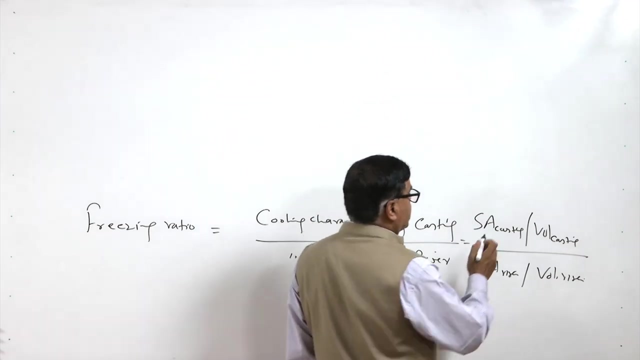 which means it is this SA, the surface area of the casting, divide by volume of the casting, divide by the surface area of the riser, divided by the volume of the riser. So this ratio has to be: surface area divide by the…. the casting solidifies first this SA surface area to the volume ratio of the casting. this 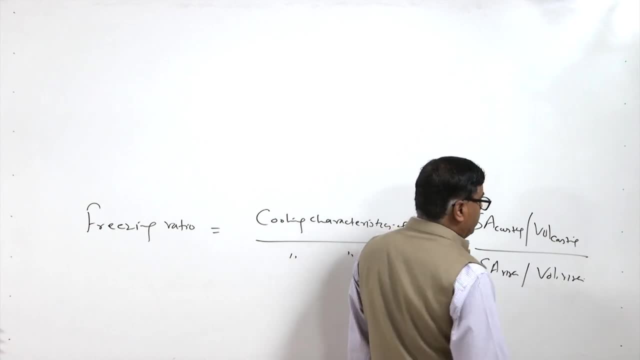 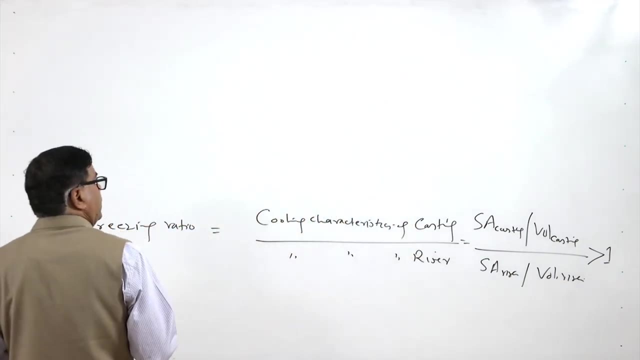 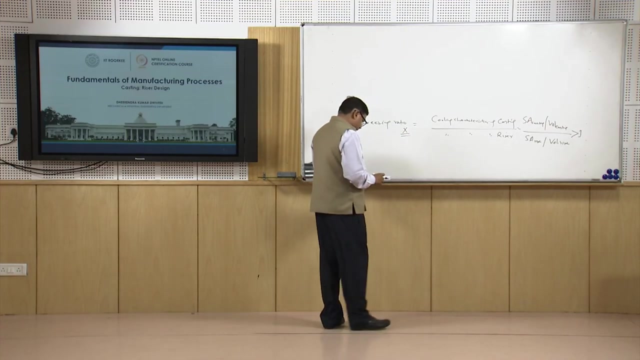 should be greater than the surface area to the volume of the riser and this ratio- that is why- should be greater than 1 in order to ensure that the riser is able to feed the molten metal to the casting. and this ratio is expressed as X, letter X. 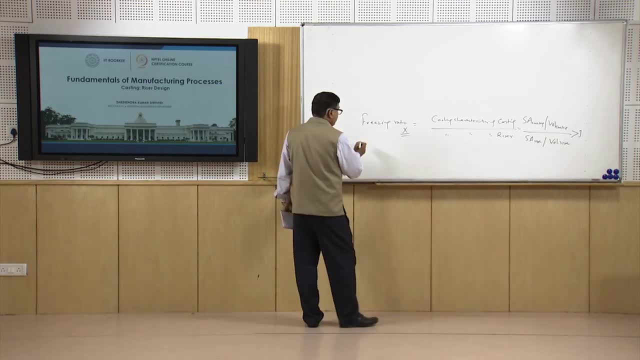 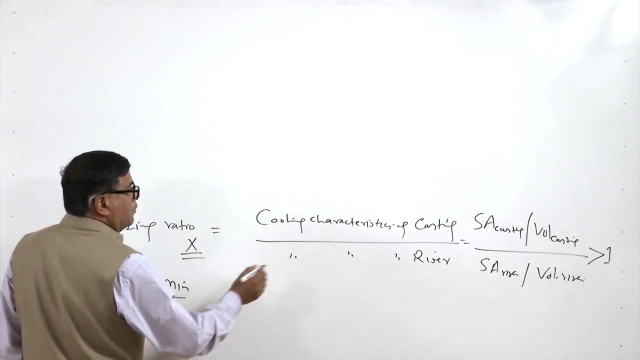 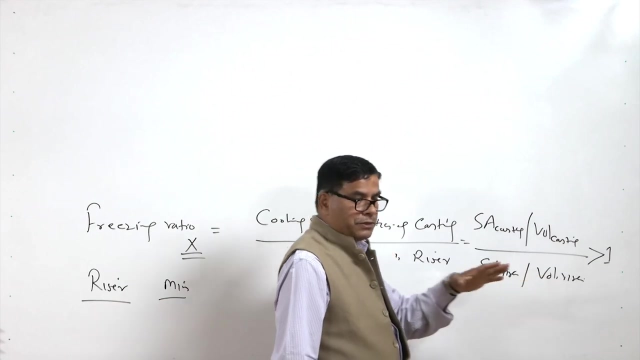 So, according to this one, what are the possible shapes for the riser, If we consider the riser with the minimum? so to have the higher value of this ratio, it is required that surface area to the volume ratio is minimum and the minimum surface area 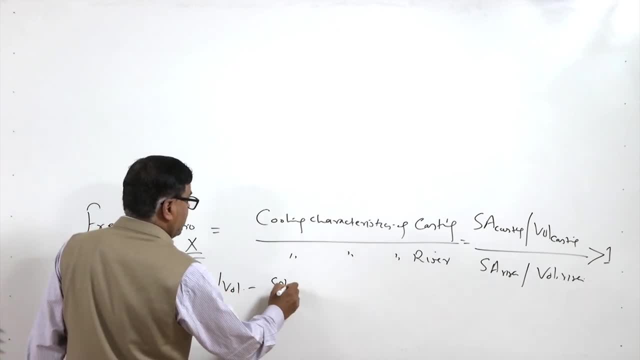 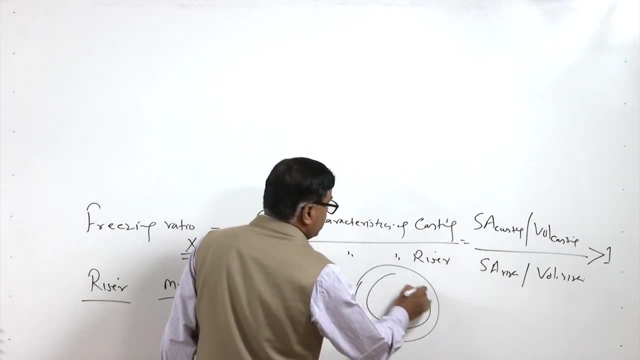 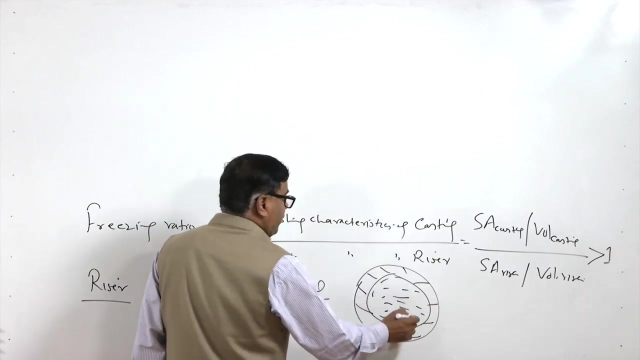 to the volume ratio. So this ratio is obtained in case of the spherical shapes. But in case of the spherical shapes, obviously the solidification will be starting from the surface and the molten metal will be left in the in between, so will not be able to. 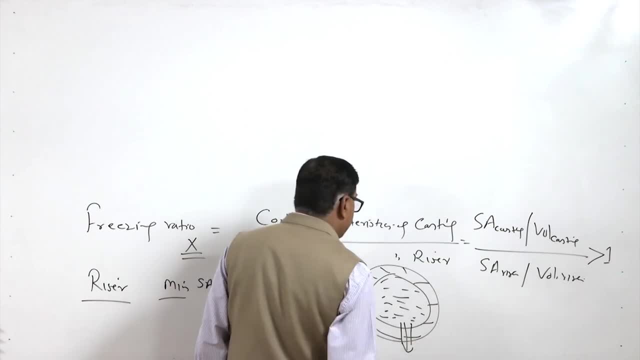 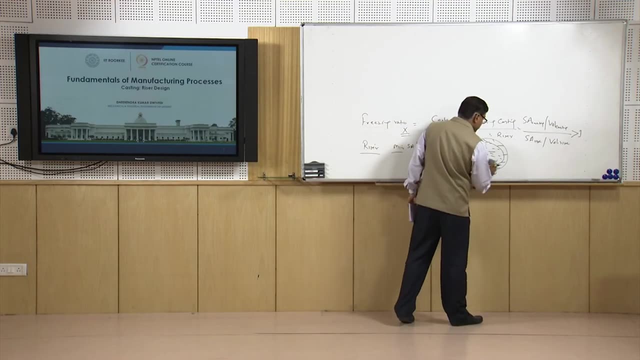 feed the molten metal from the riser to the mould when it is desired. So this is found to be difficult to implement for using as a riser shape. So next preferred shape. So the preferred shape for the riser is the cylinder. So in case of the cylindrical shape risers, basically the length and the diameter of the riser is obtained as far as the design is concerned. So, basically, efforts are made to determine the diameter and the length of the riser so that the desired freezing ratio can be determined. 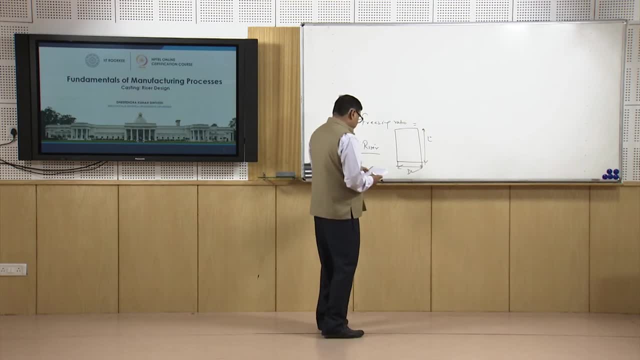 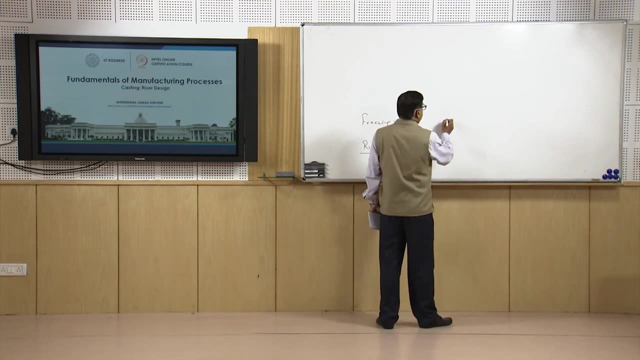 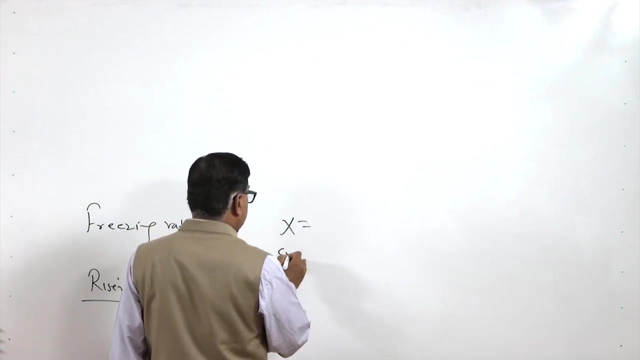 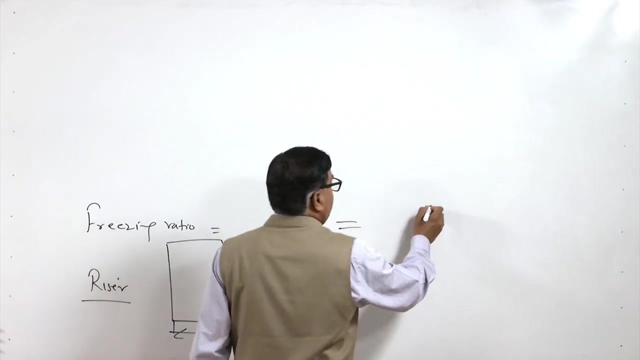 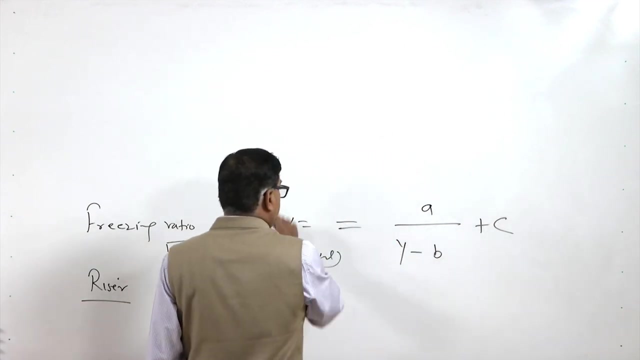 Ok, So here some freezing ratios for the cylindrical shapes have been. equations have been developed for obtaining the freezing ratios for the risers of the cylindrical shapes. Cylindrical shapes: this is expressed as A by y minus B plus C. this is one typical freeze. 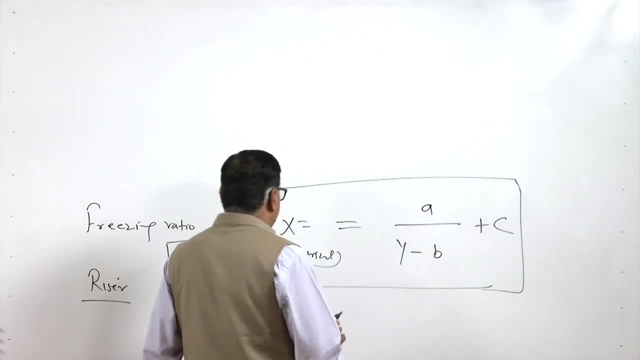 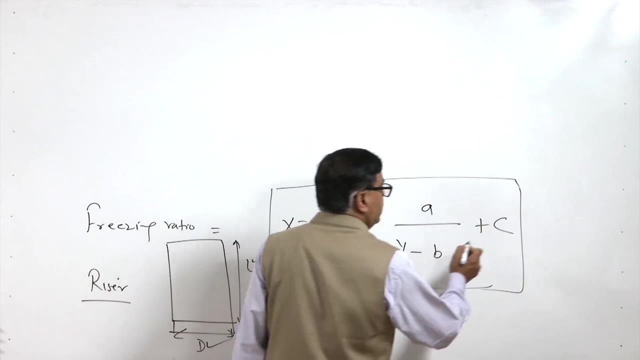 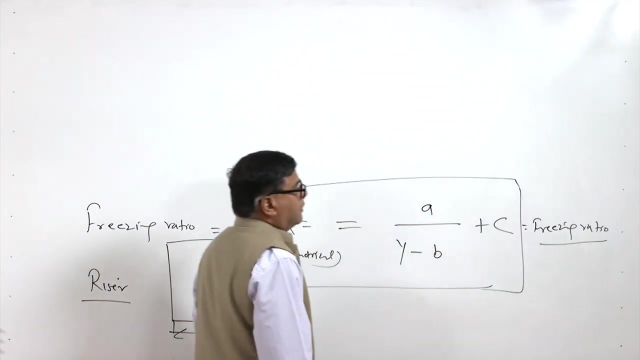 equation used for determining the freezing ratio for the cylindrical shape risers. So where this, as I have already told, this is basically the freezing ratio, which is the ratio of the characteristics of the casting to that of the riser, and the Y is the ratio of the riser. 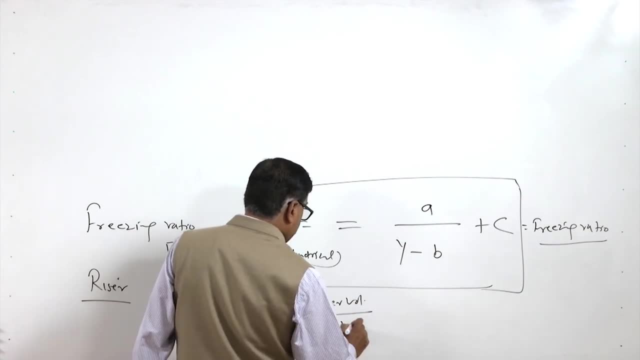 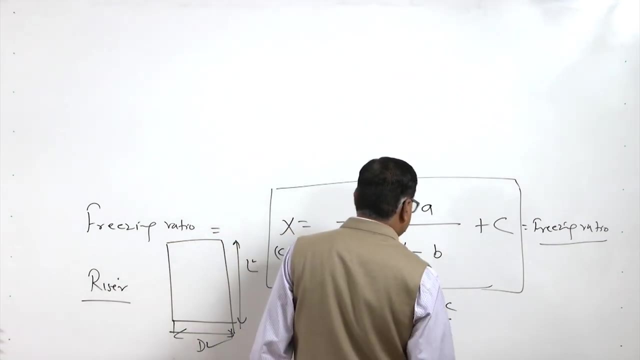 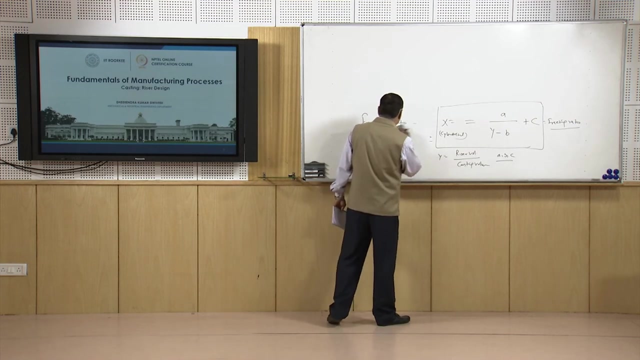 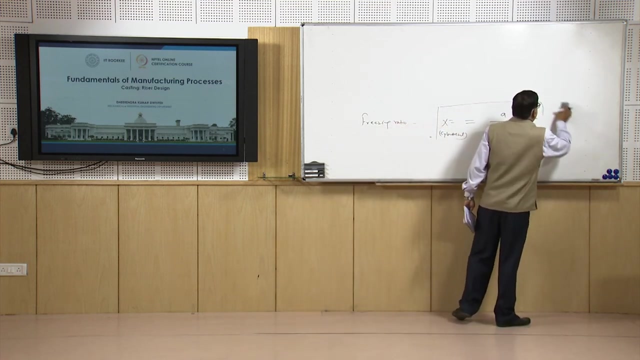 volume to the casting volume and A, B, C are basically A, B, C are the constant. So people have developed the identified the value of the constants through the experimentation for designing the risers. So here I will be writing that values of the common constants which are used for designing 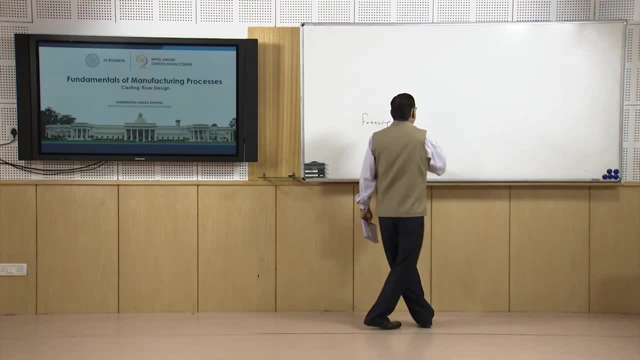 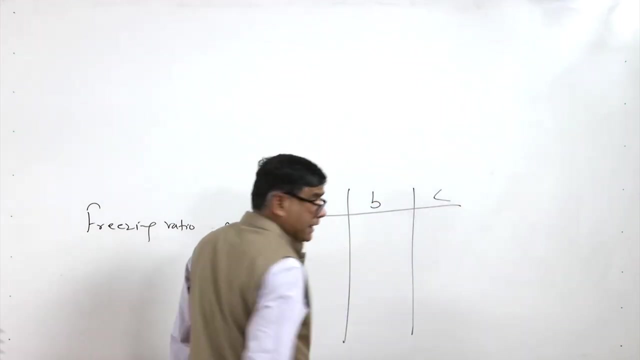 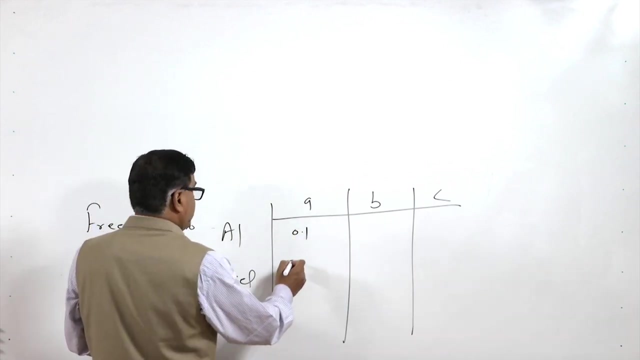 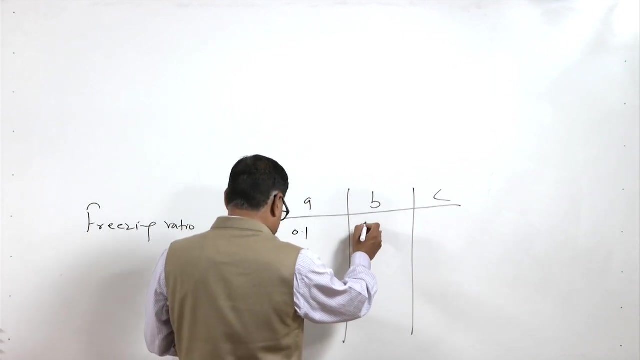 the risers for the common foundry metals, Say for aluminium, steel and cast iron, the values of A, B, C are the constant values. So like A for aluminium 0.1, for steel 0.1 and for cast iron 0.04 and B for aluminium. 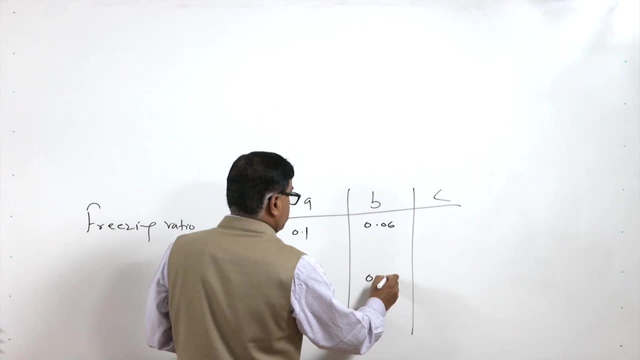 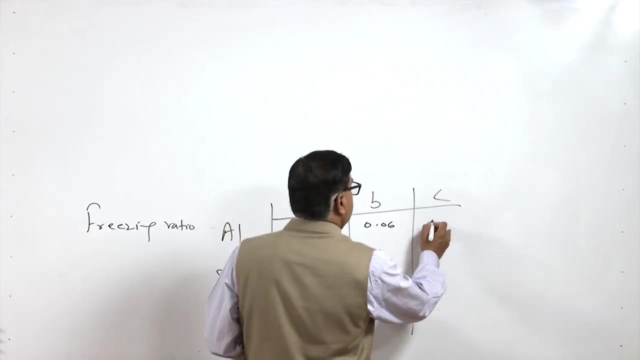 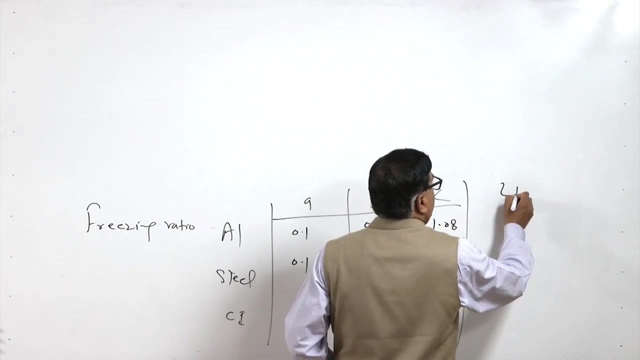 is 0.06, 0.03 for steel and 0.017 for cast iron. Similarly, C for aluminium is 1.08, 1 and 1 for cast iron. One typical freezing ratio for one of the commonly used aluminium alloy: LM4 freezing. 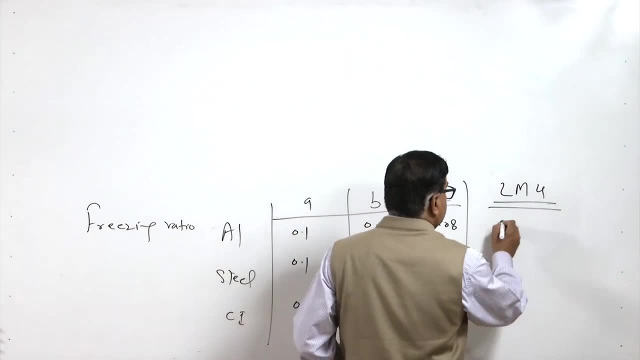 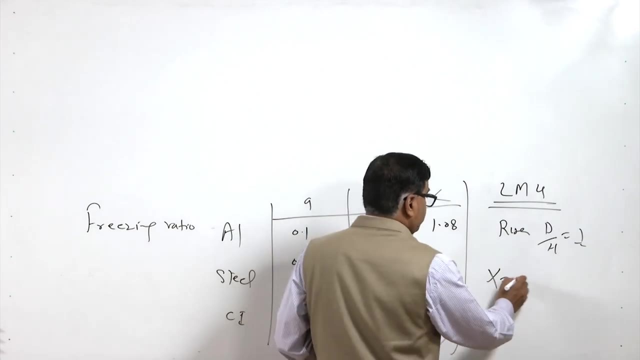 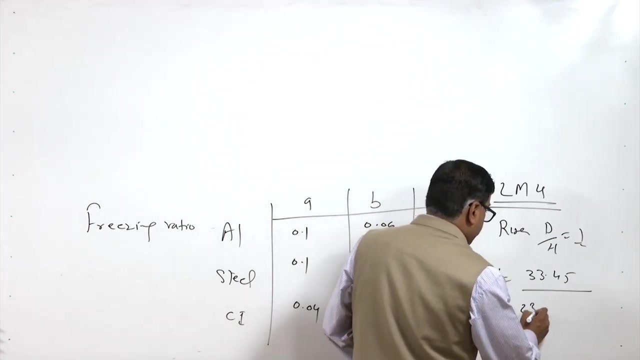 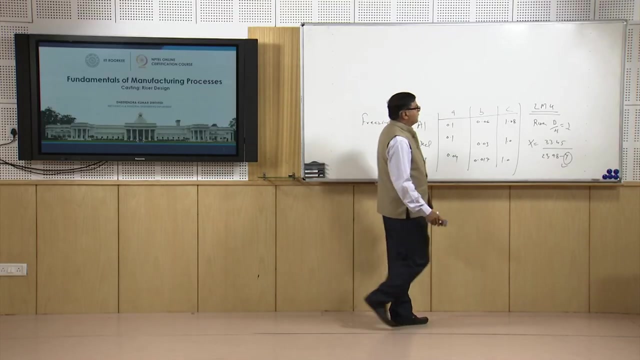 ratio for the riser. when the diameter to the height ratio is 1,, the freezing ratio is given by the equation 33.45 divided by 23.98 minus y. So this, basically the y, is used for determining the volume of the riser, while considering: 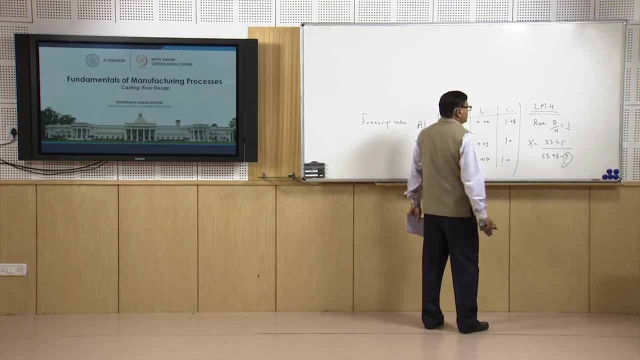 the. this ratio d by h is equal to 1, means the diameter to the height ratio of the riser is 1.. So this is 1.. Since it is always desired that the value of x is greater than 1 in order to ensure: 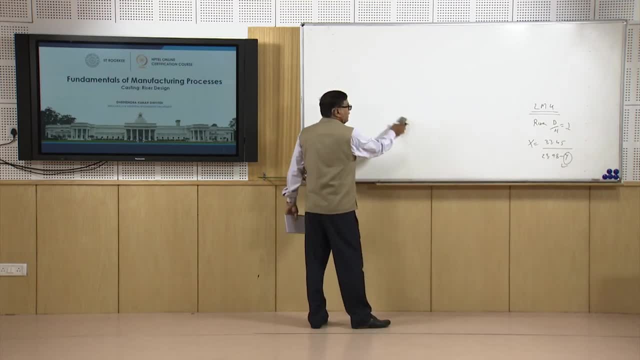 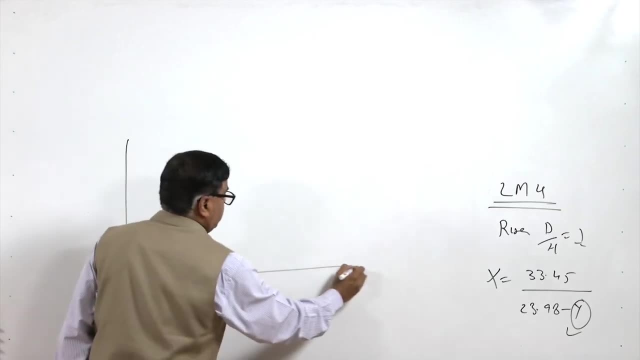 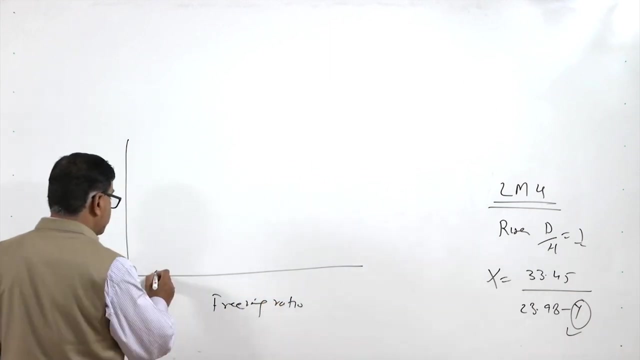 that the molten metal in the riser solidifies at the end. we will be now seeing one typical plot which shows the relationship between the freezing ratio, which should be greater than 1.. So freezing ratios from 1 to say 1.9 at the interval of, say, 1.9.. 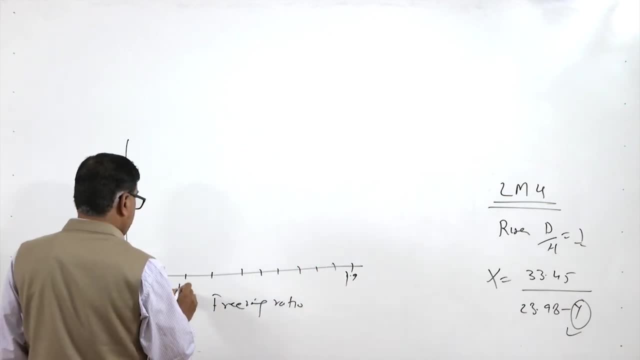 So that means this rate and exercise u delay can say 0.1,, we can say so 1, 1.1,, 1.2,, 1.3, and likewise to 1.9, and here the volume of the riser to the volume of the casting. 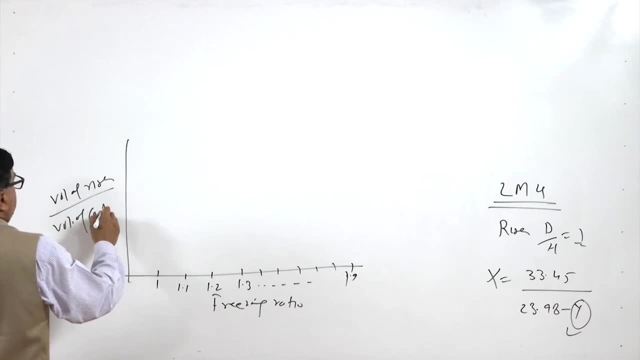 This is basically the value of the y in our equation. So the relations between, basically, the x and the riser will have given the remaining for further discussion. So we have discussed this. Now what is tomorrow? we can discuss tomorrow x and the y and what it shows, that it goes in like this: here the value of the y is in: 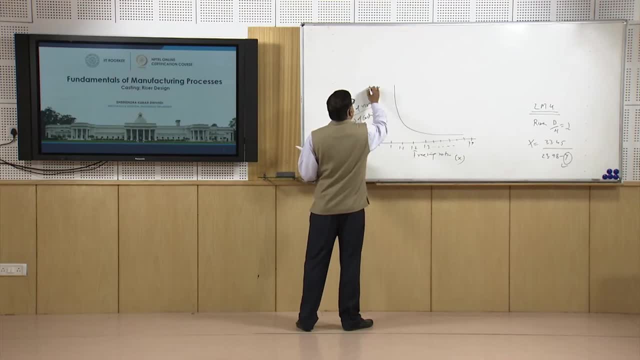 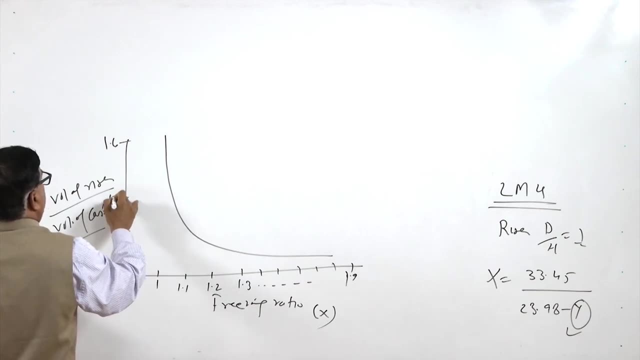 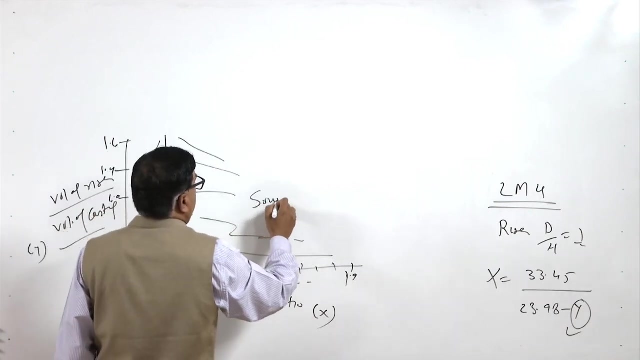 the range of like, say, 0.2 to 1.6, 0.6, 1, 1.4, like this, And what we see here when this the freezing ratio is greater than 1, and this so the there are 2 zones. basically, this line divides the 2 zones. one is the sound casting and another. 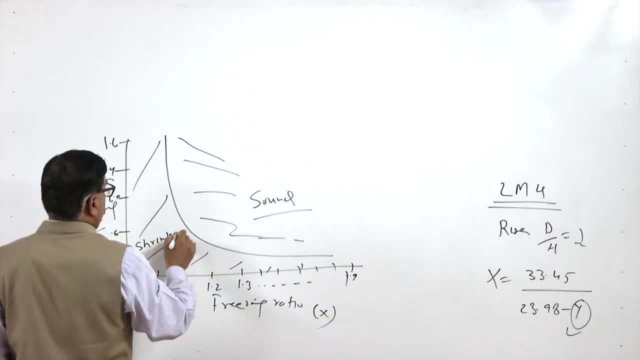 is, with the shrinkage porosity, So proper. the values of the y and x are different, To be maintained in order to have the sound casting. and if the 2 are not maintained, like say, what should be the freezing ratio for the different values of the y and what should? 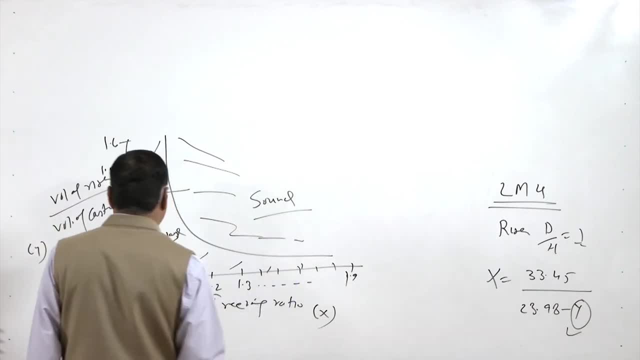 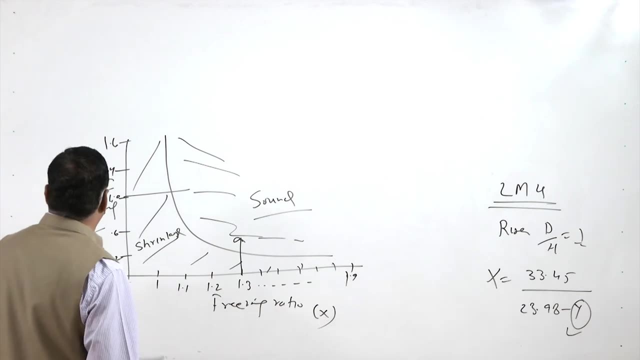 be the value of the y for the different freezing ratios. that is what can be obtained. So if the freezing ratio is high, then even the low riser to the volume of the casting can be used, And if this kind of ratios are used, then these will be helping. 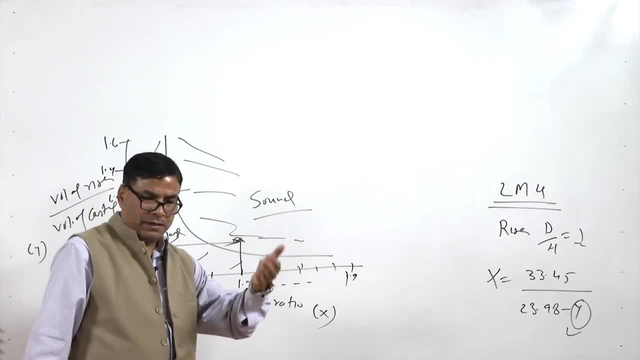 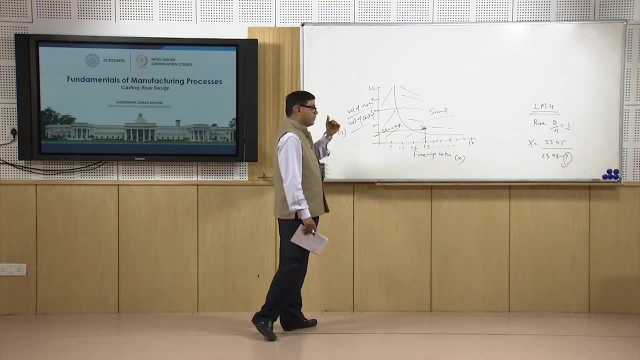 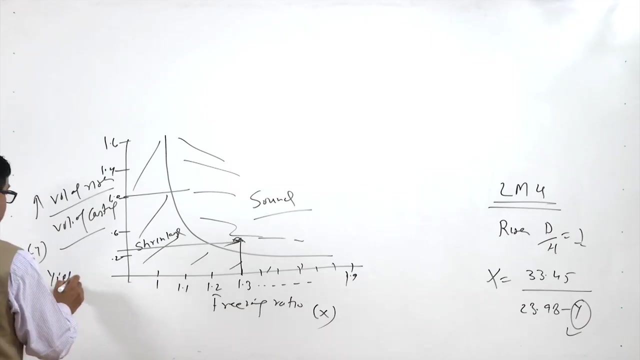 In increasing the yield because the ratio of the molten ratio of the riser- molten metal in the riser- to the ratio to the volume of the metal in the casting. So if this ratio is high for sound casting then definitely our yield will be much better. 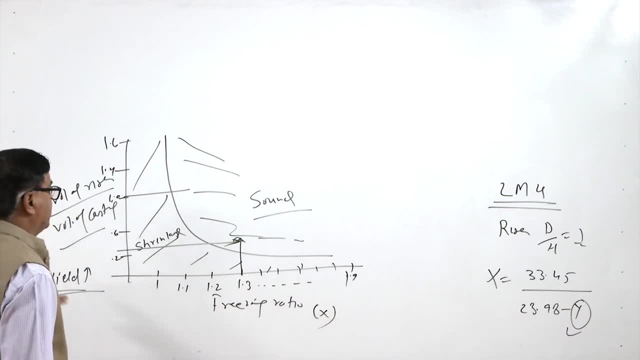 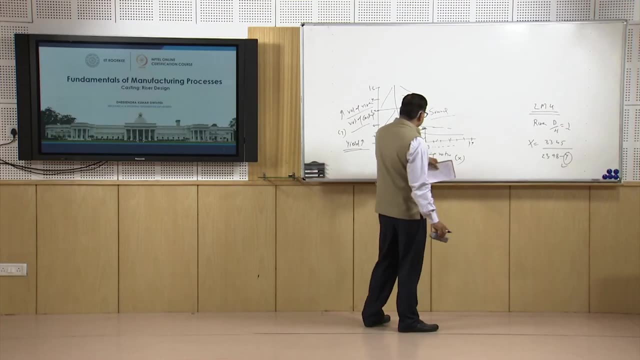 because in molten metal being solidified in the riser that will be less as compared to the volume of the metal which is solidifying in the casting. So efforts are always made So it is better to have the much better freezing ratios for using the high for achieving the 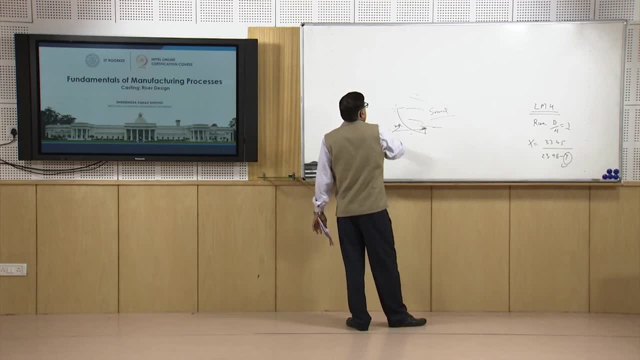 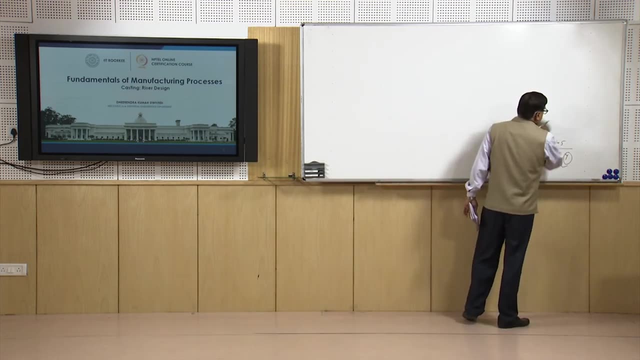 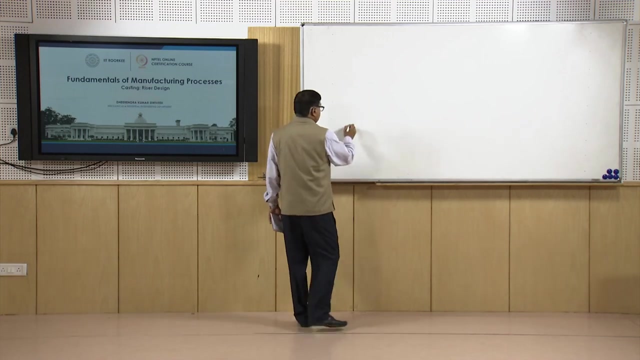 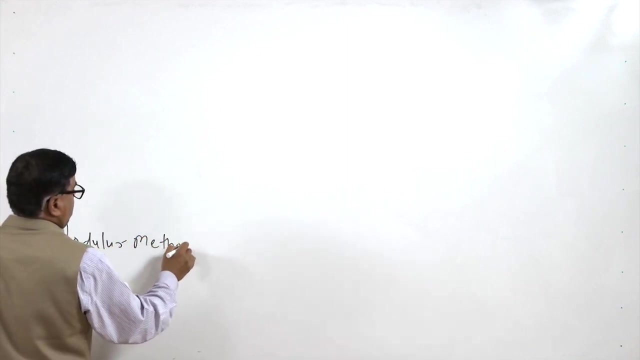 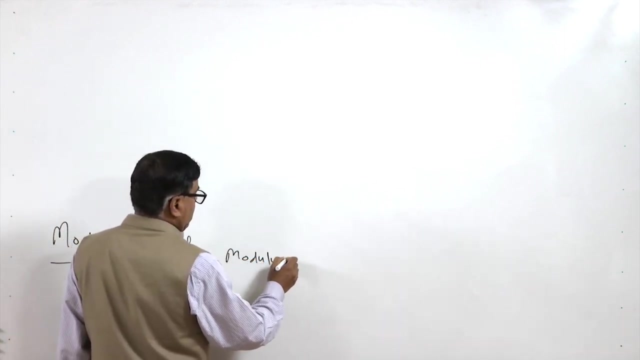 high yield through the low riser volume to the casting volume ratio. There is another method of the riser design and that is called modulus method: Modulus, Modulus, Modulus, Modulus, Modulus, Modulus method. This basically determines the modulus of casting and modulus of the riser. 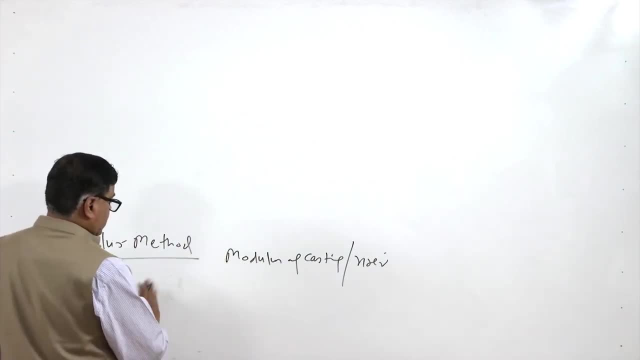 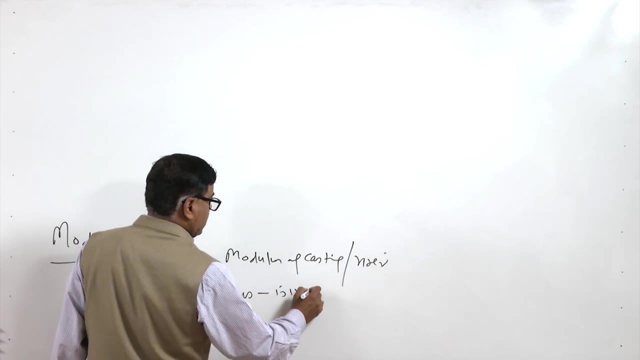 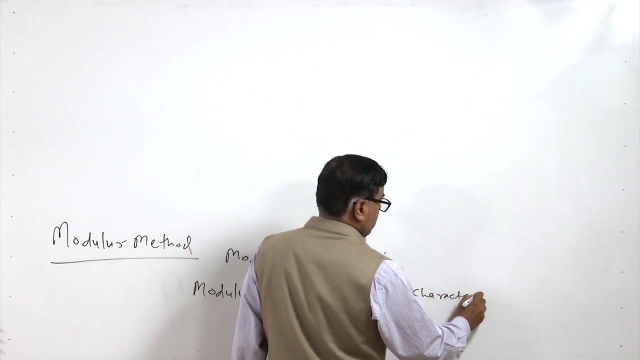 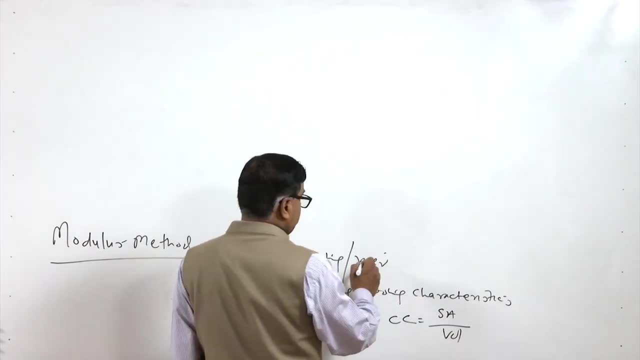 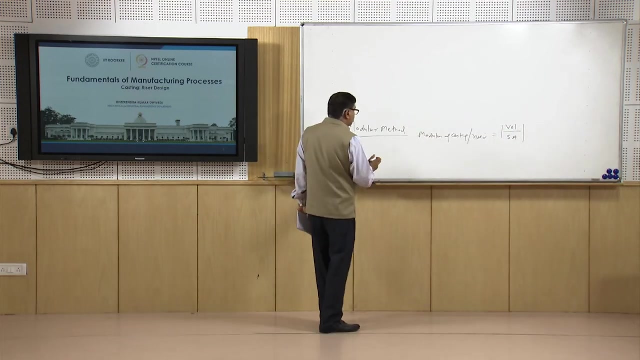 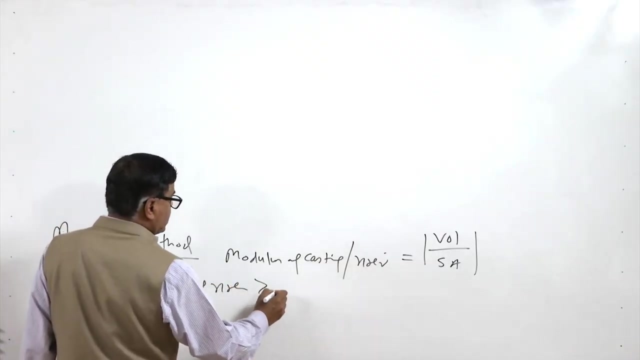 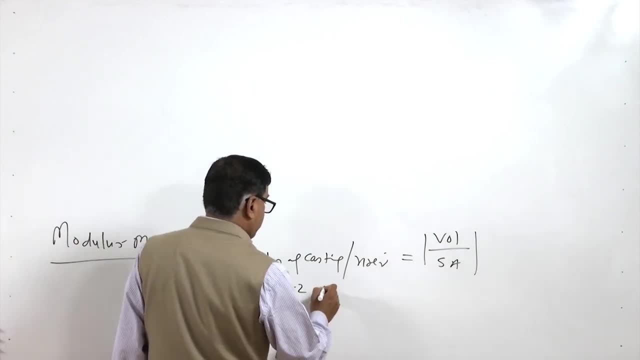 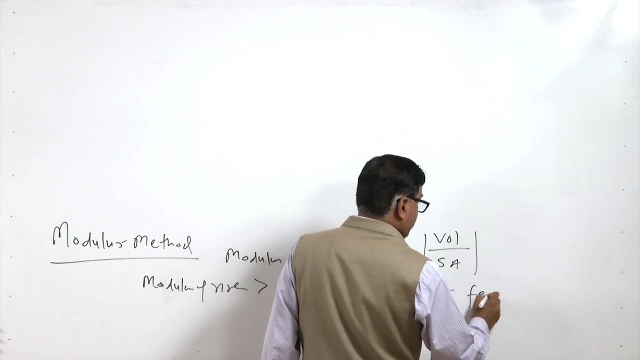 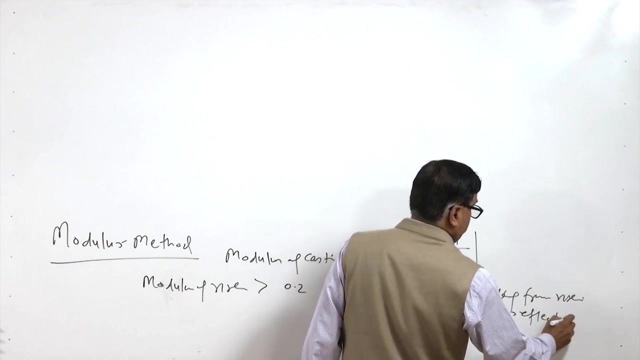 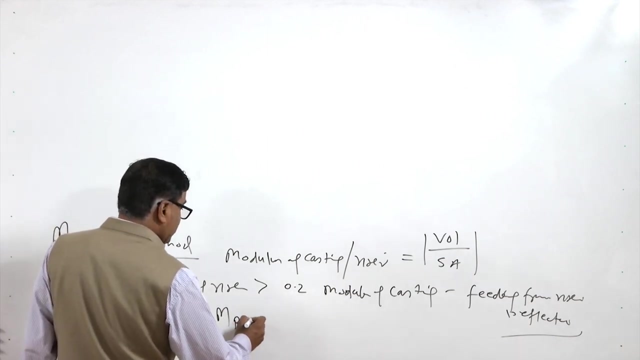 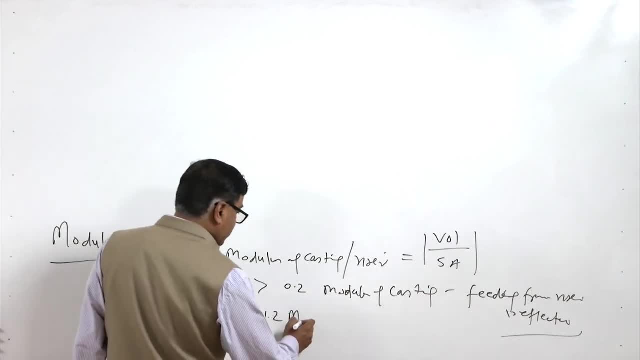 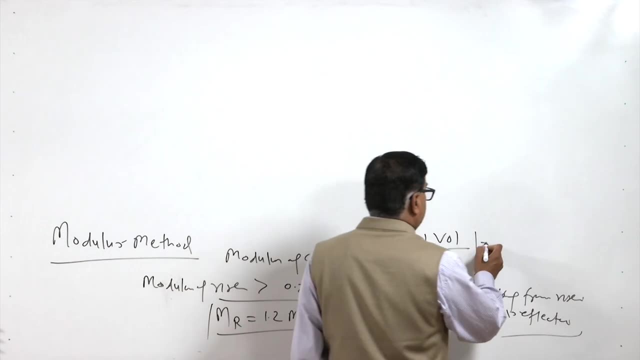 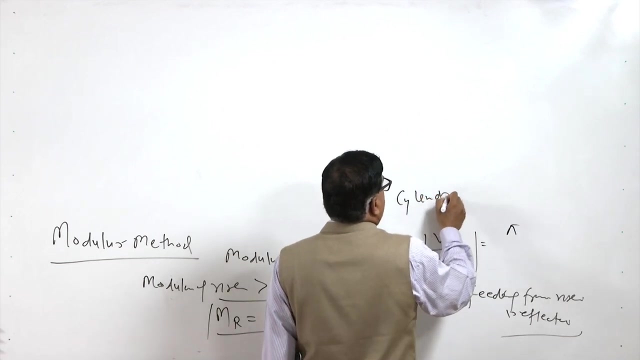 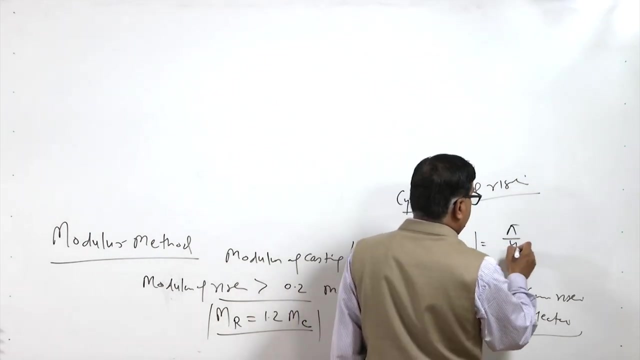 equal to 1.5, 1.2 times of the modulus of the casting. this is what is to be maintained. So if we go by this, then it comes out to be the volume of the volume of the casting. say, for cylindrical riser or casting, the volume is like pi by 4, D square into L. L is the 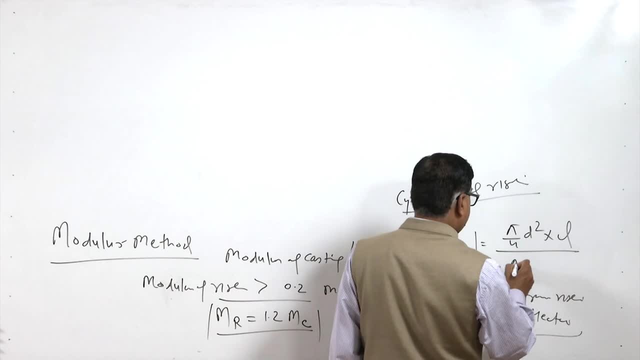 length and D is the diameter divided by surface area is pi D into L. So here L and L will be cancelled, D and D will be cancelled. So here 1, D is left, pi and pi will be cancelled, will be cancelled. So we are left with the d by 4.. So which is precisely 0.25 d mostly. 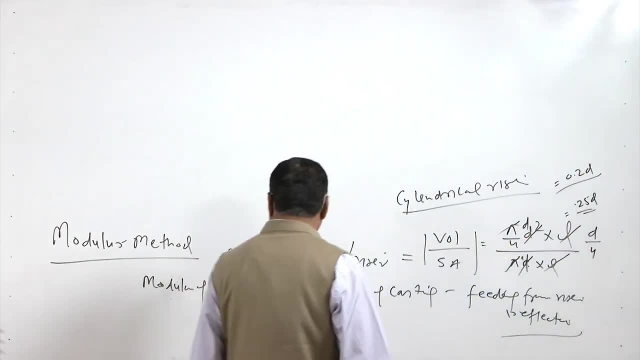 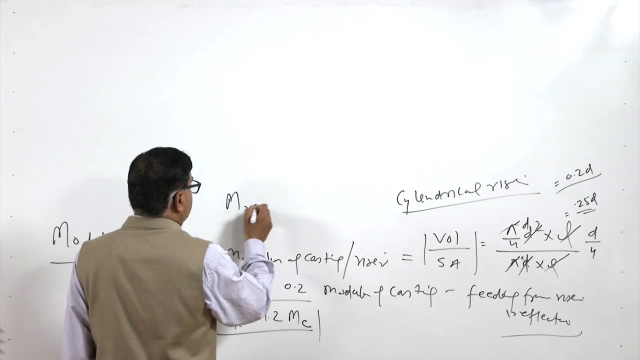 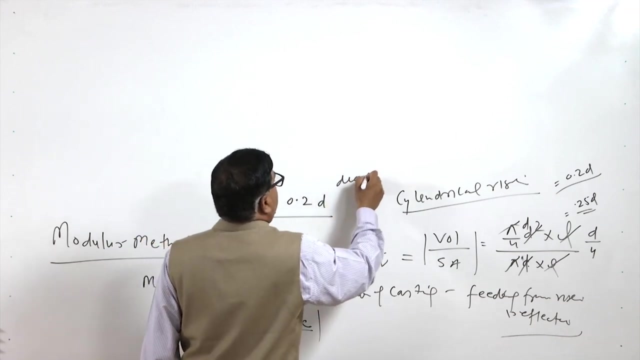 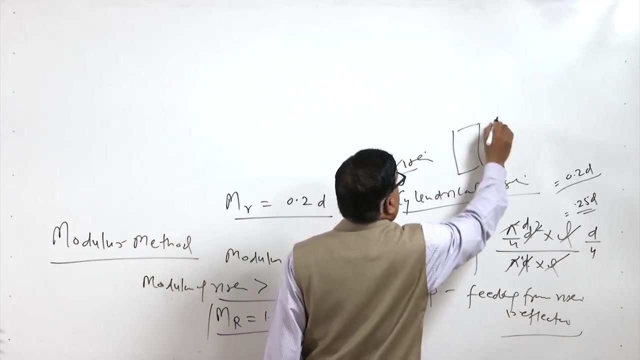 it is taken as 0.2 d. So if you have to determine modulus is basically modulus of the riser is 0.2 times of the d. D is the dia of diameter of the riser if it is the cylindrical riser.